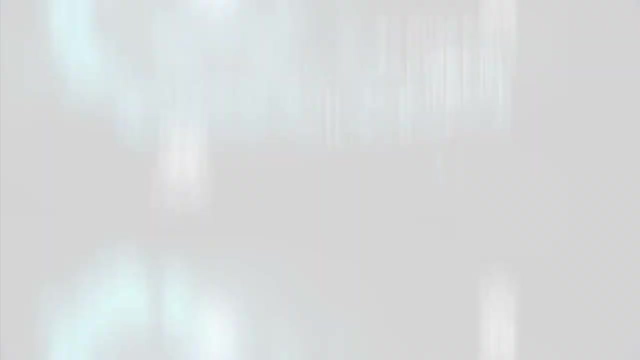 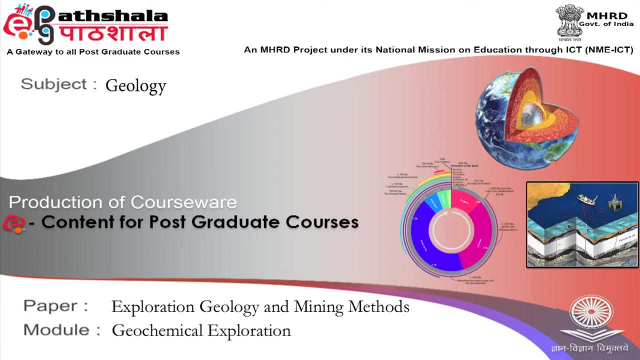 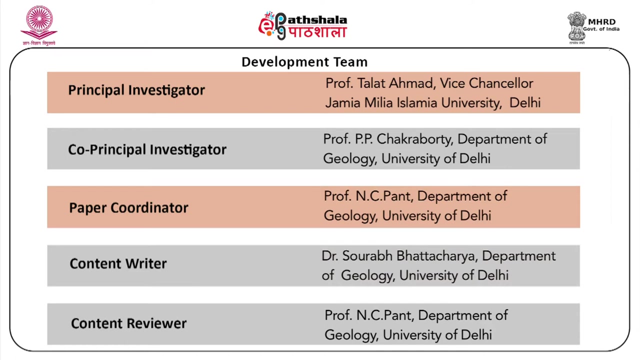 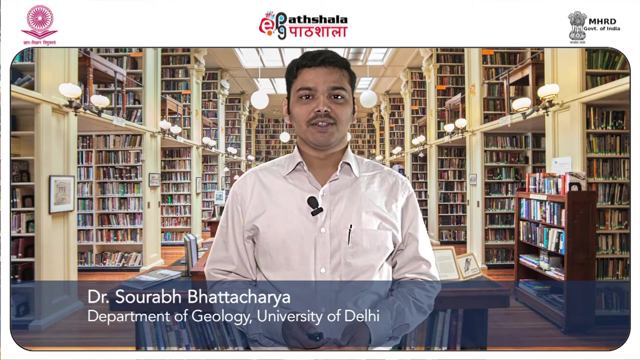 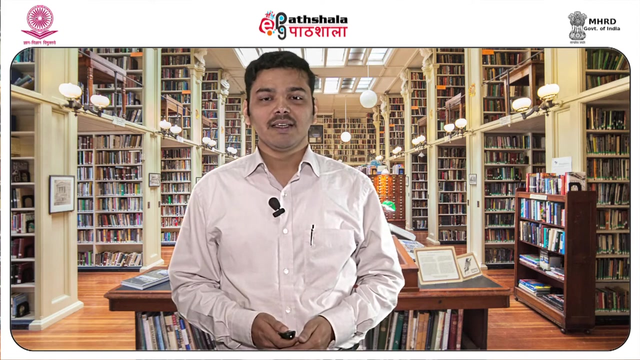 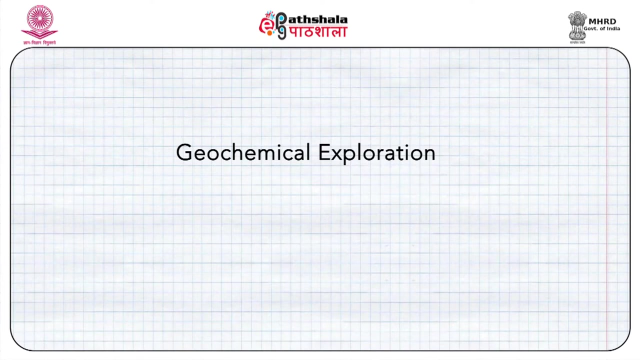 Hello students, I am Dr Soro Bhattacharya from Department of Geology University of Delhi. I hope you are going through other modules in geology. The present module I am going to discuss today is on geochemical exploration. After studying this module, you shall be able to: 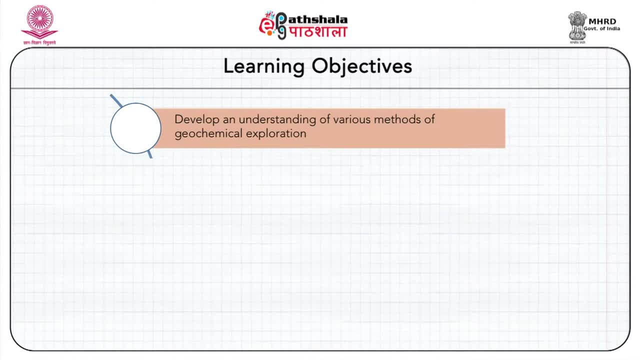 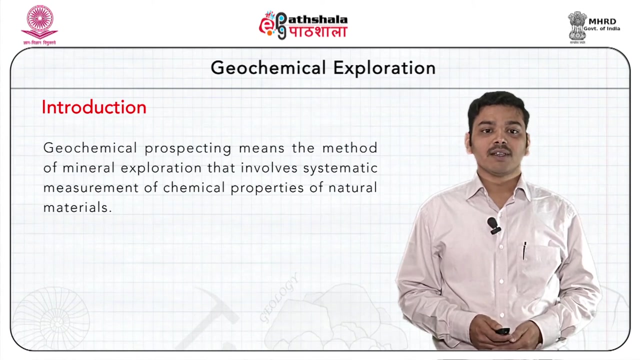 develop an understanding on various methods of geochemical exploration. Also, you shall be able to appreciate the importance of dispersion patterns of elements in geochemical exploration. Geochemical prospecting means the method of mineral exploration that involves systematic measurement of chemical properties of natural materials. Mostly, we are interested in measuring 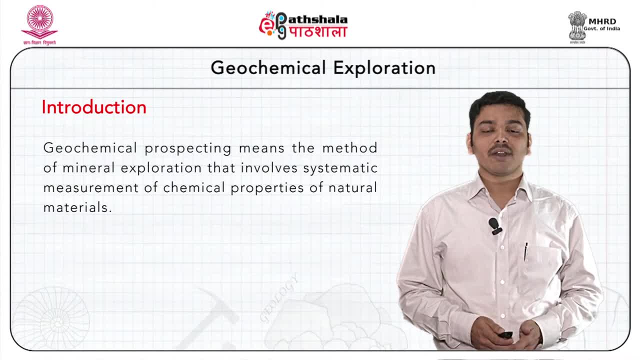 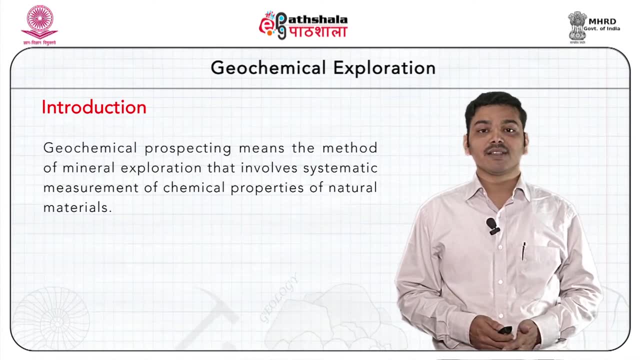 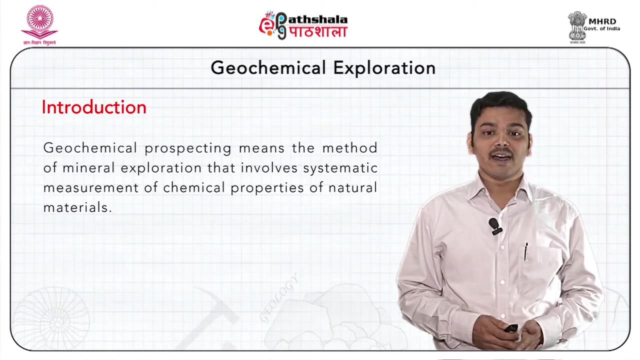 the trace amounts of any element or a group of elements. The purpose of any such exploration is to discover a geochemical anomaly, which means a chemical pattern in an area indicating presence of ore in proximities. Mineral exploration essentially involves practical application of principles of geochemistry constraining the abundance of 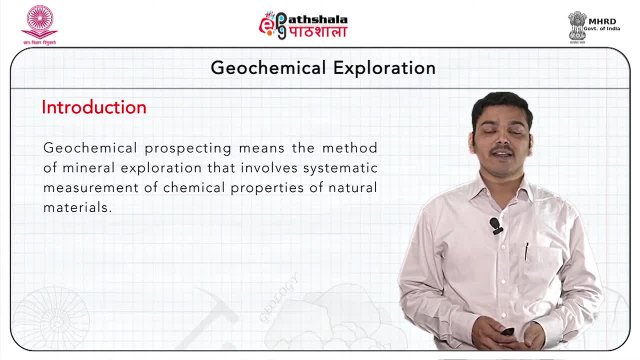 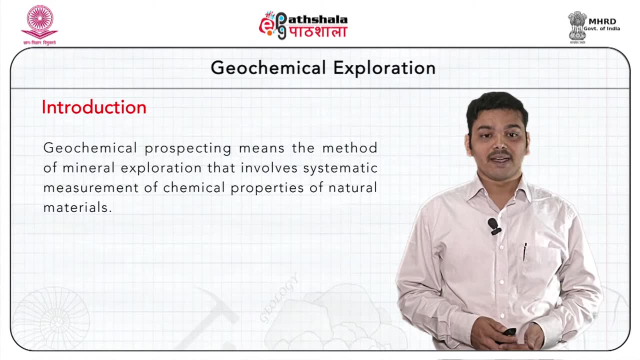 certain elements in geochemical exploration. The purpose of mineral exploration is to discover a geochemical anomaly in an area indicating reference to a geochemical evidence related to a geochemical level or distortionット. Part 2: The depth at which geochemical adsorption events in earth materials and recognition of geochemical 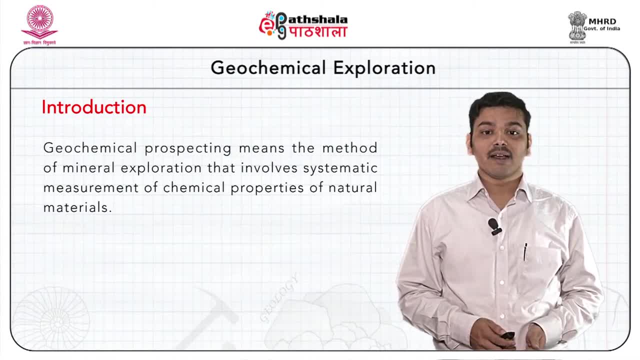 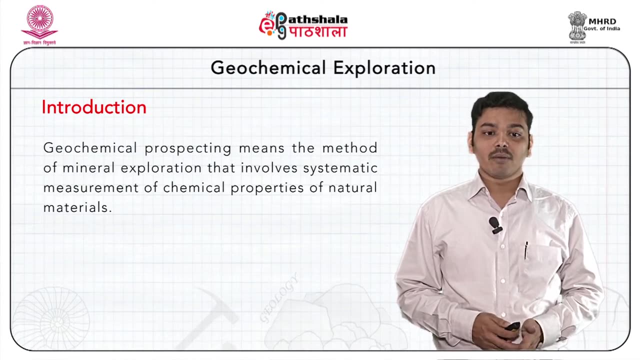 anomalies in space is critical for prospecting. Often such anomalies reflect unusual concentration of commercially-critical elements identified when compared with areas lacking mineralization. Background is the term referred for normal concentration of an element in geosynthetic and pulsezed ownership. Use of geosynthetic elements often means the below 2,000 film chromatic. 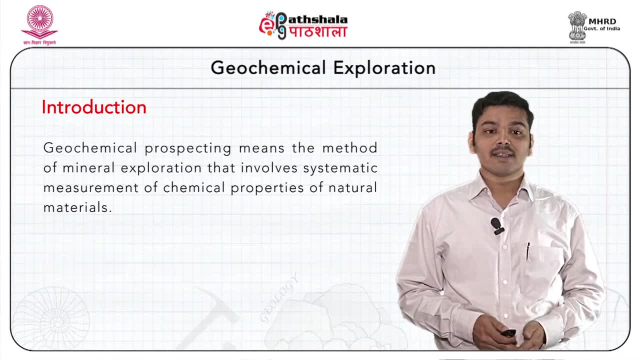 in natural material, where the equilibrium has not been disturbed by ore enrichment processes, Background values may have a broad range. in result to physicochemical processes causing enrichment of certain elements and depletion of others, A state of fluidity is attained which facilitates recrystallization and differentiation of several varieties of igneous. 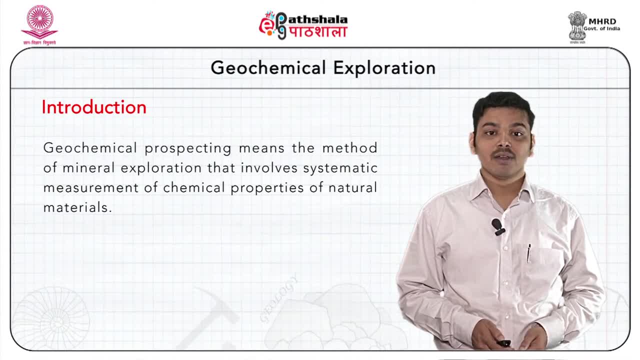 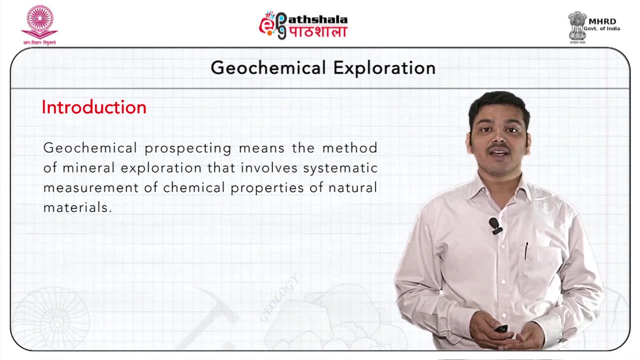 rocks and related hydrothermal rocks. Further erosive processes expose such rocks and bring them into surficial conditions. Thus the various components of the rocks are resorted due to action of weathering agencies. Hence a new series of sedimentary rocks are deposited. closing. 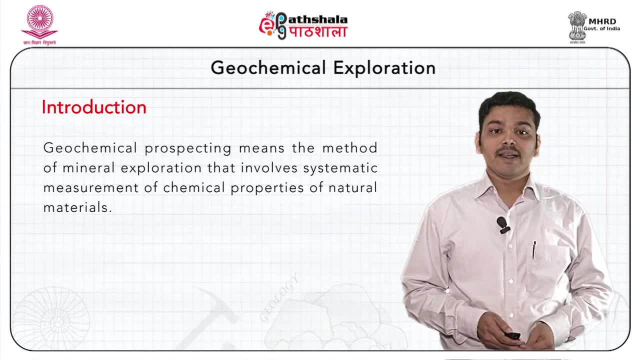 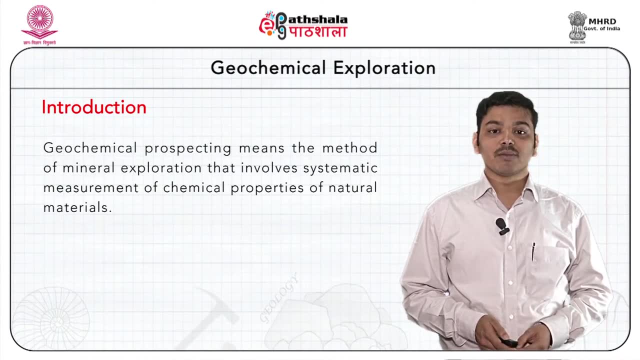 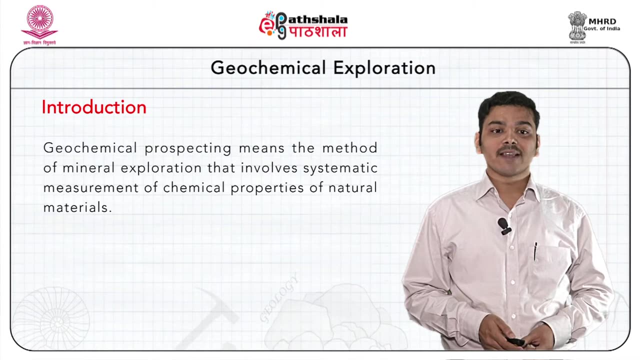 down and re-exported to other areas of the world. These rocks are then re-exported to other areas of the world. For example, it is common for sedimentary rocks like sandstone and shale to escape the metamorphic transformation. rather are exposed for weathering and erosion. The overall cycle comprises two parts. 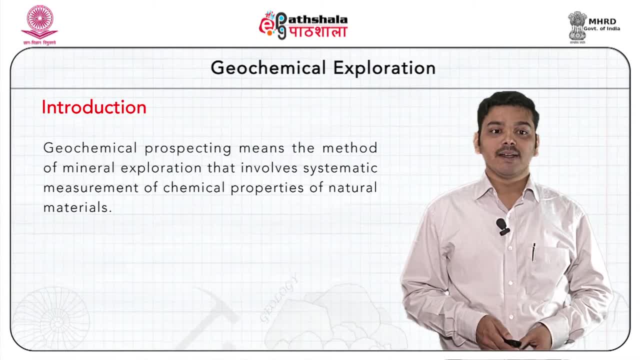 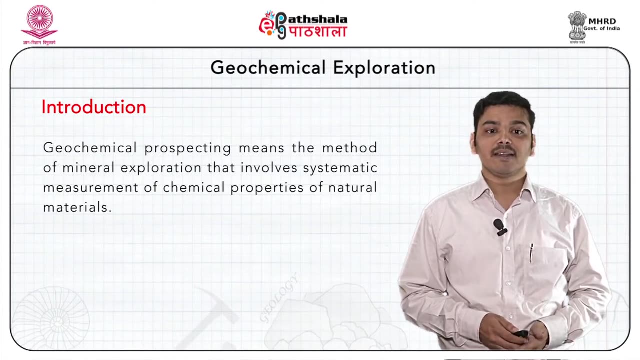 One takes into account the deep-seated processes of metamorphism and igneous differentiation. The other highlights surficial processes of weathering, transportation or sedimentation. The horizontal division marks the boundary between these two phases of geochemical cycle inside the rock. 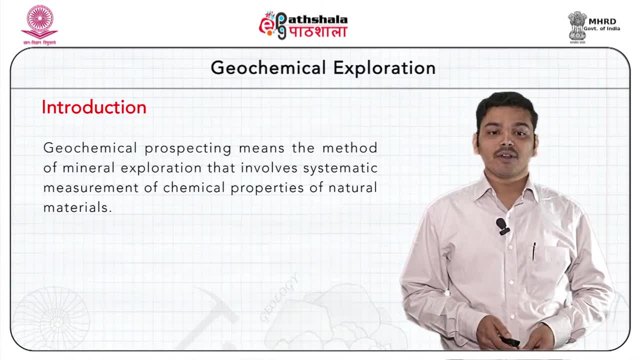 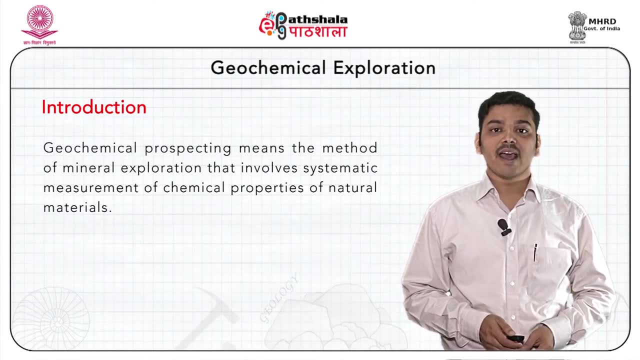 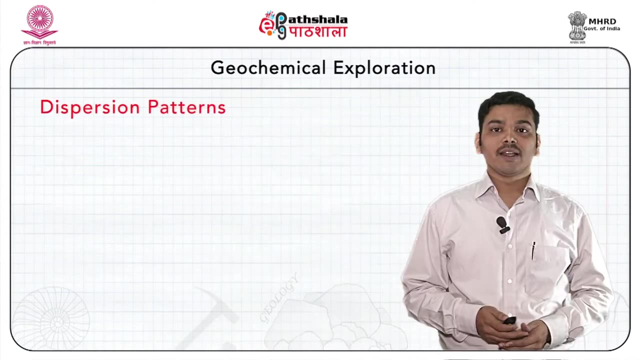 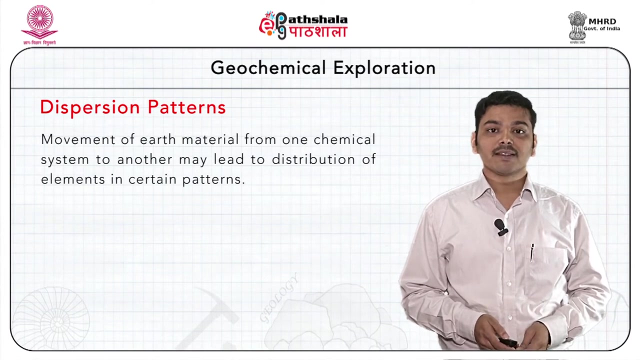 You may see in Figure 1,, Petrology and Economic geologist refer to deep-seated and surficial processes as endogenetic and exog fundamentalist respectively. So the next section is on dispersion patterns. Movement of earth material from one chemical system to another may lead to distribution of 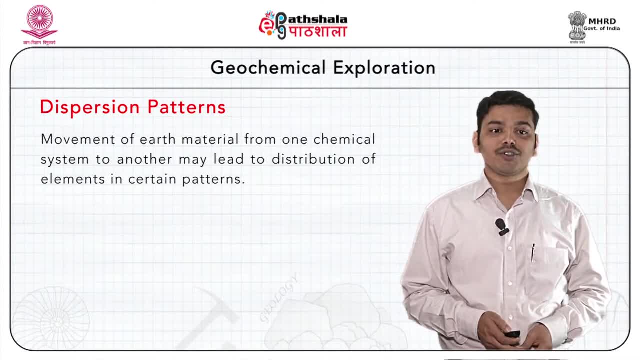 elements in certain patterns. Such distribution patterns reflect the abundance of elements in the moving material and chemical equilibria characteristic of the local environment. This distribution pattern of elements is referred as dispersion pattern, a term signifying the dynamic processes involved in their formation. Dispersion pattern occur as areas where abundance 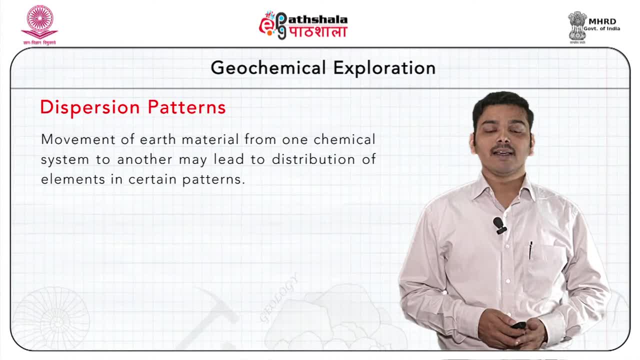 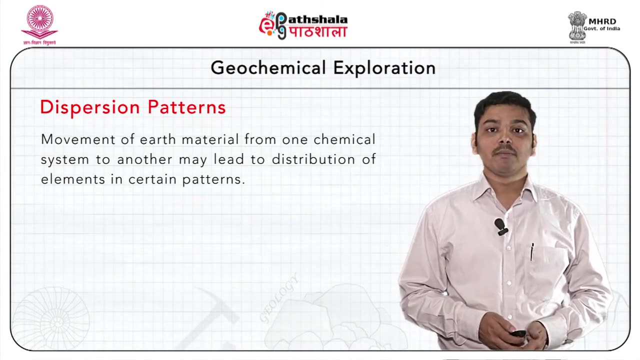 of any particular element is higher than in the surroundings. They are the result of local enrichment of elements in higher than average amount. The dispersion patterns are helpful in mineral exploration if the enriched source is an ore deposit or else is related to ore formation. Thus dispersion pattern can also be regarded as a geochemical anomaly. 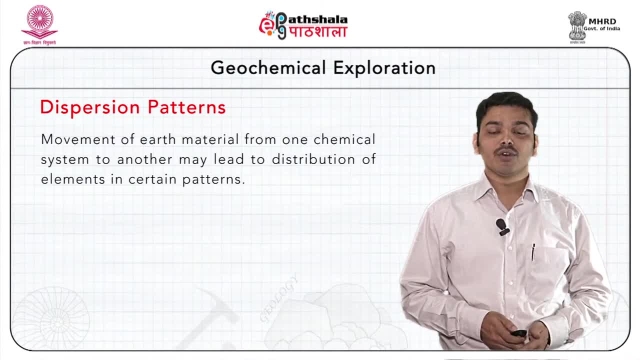 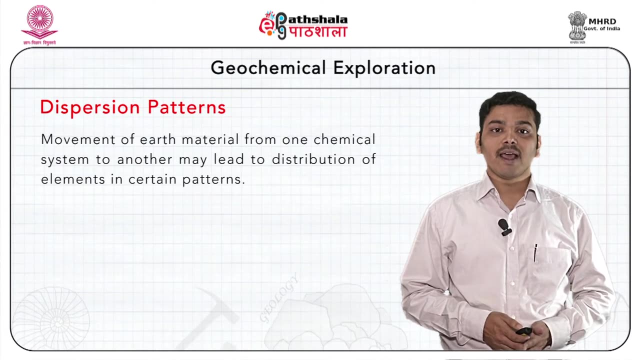 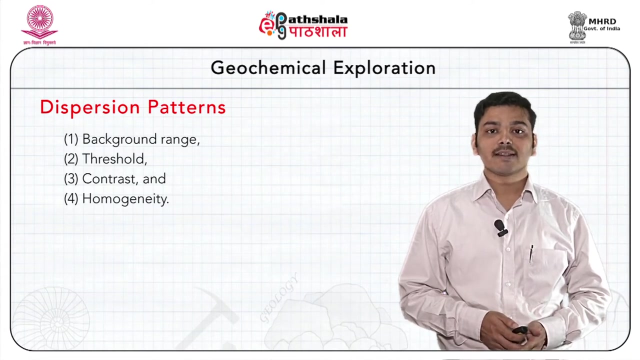 It is very important to distinguish geochemical anomalies from dispersion patterns of no economic importance. Some of the empirical parameters that are critical to identify and interpret geochemical anomalies are: first, background range, second, threshold, third, contrast and fourth, homogeneity. Background range means the well-defined range of geochemical data in areas where the equilibrium has 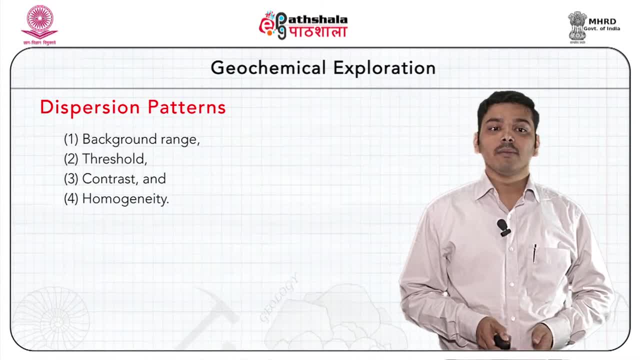 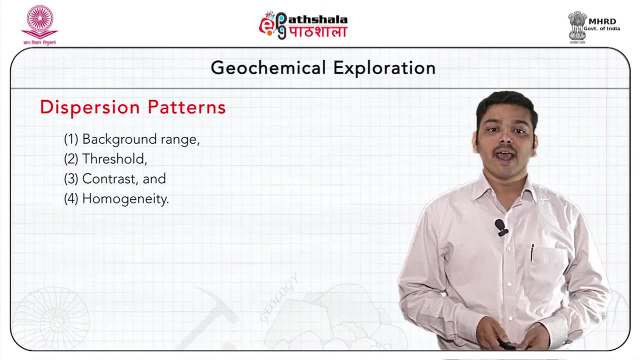 not been upset by the presence of a mineral deposit. During interpretation of geochemical patterns in an area showing anomalies, it is usually possible to choose a certain limiting cutoff or threshold value below which the variations show just normal background effects, And above these variations are significant variations of geochemical patterns, such as geochemical 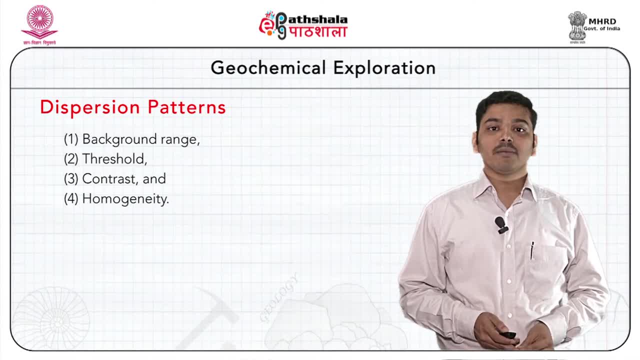 relief or contrast in an area showing anomalies. These variations are significant by means of a possible ore deposit. In interpretation of geochemical data in terms of mineralization, contrast is a qualitative measure of the probable importance of an anomalous area. One of the criteria to judge the importance of an anomaly. 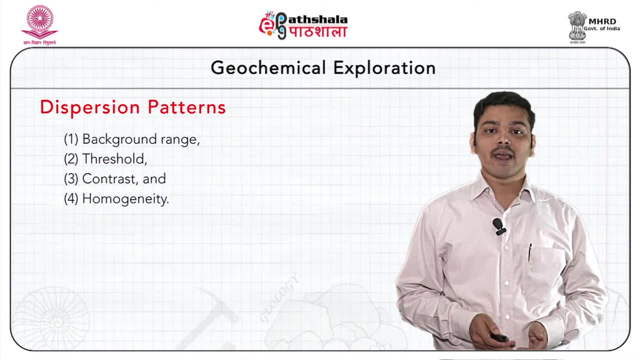 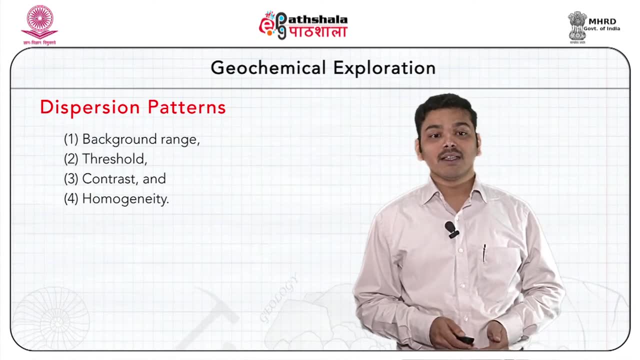 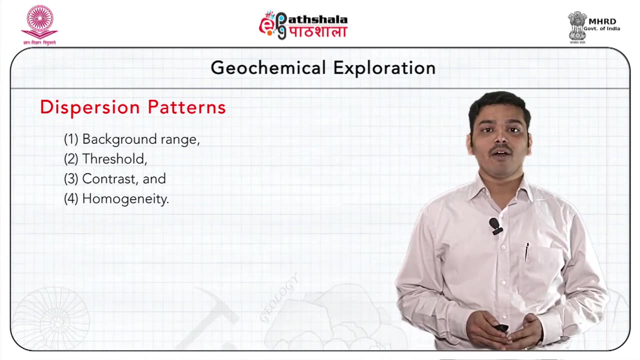 is the geochemical relief or contrast among anomalous and background values. This can be produced with the help of a Nu. This contrast may be indicated as ratio of either of maximum to threshold, maximum to background or threshold to background, depending on which numeric value appears to be meaningful. 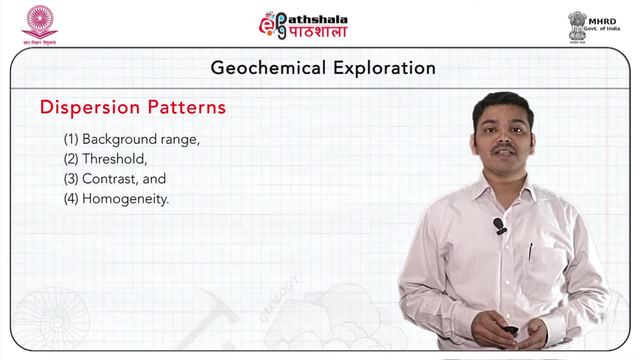 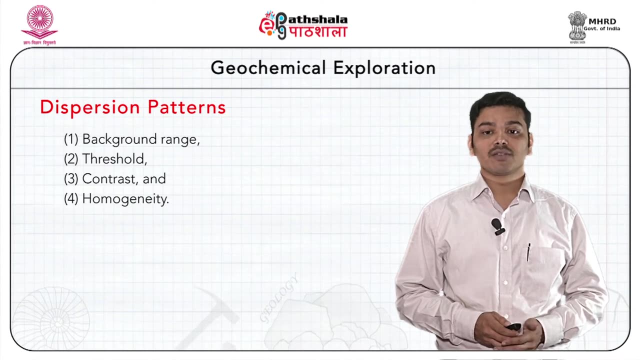 The homogeneity of a geochemical anomaly is a measure of the evenness in the distribution of the indicator mineral. For a homogeneous, anomalous area, geochemical profile contours would be smooth. In an area of inhomogeneous, anomaly, values vary radically through a wide range within. 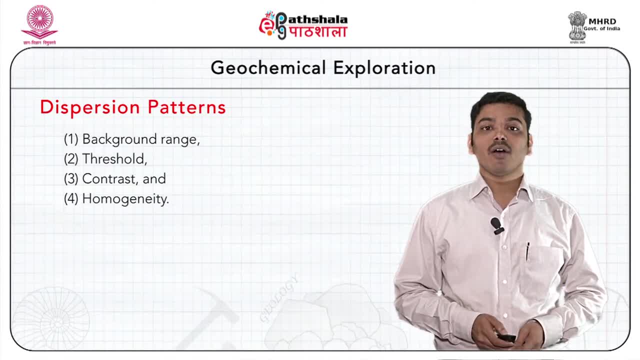 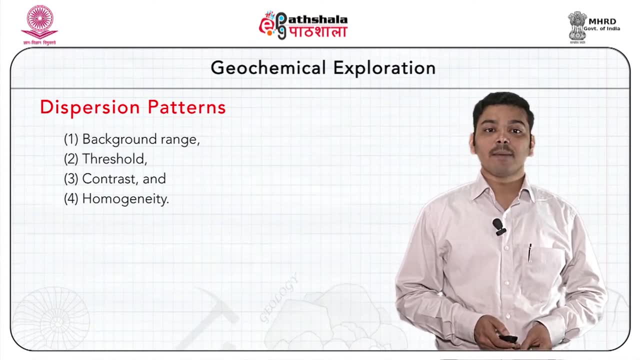 short distances. The homogeneity of an anomaly is one of the main concerns to decide for optimum spacing of samples for a geochemical survey, Based on the depth at which dispersion patterns are generated, they are classified as primary or secondary, as I am going to describe next. 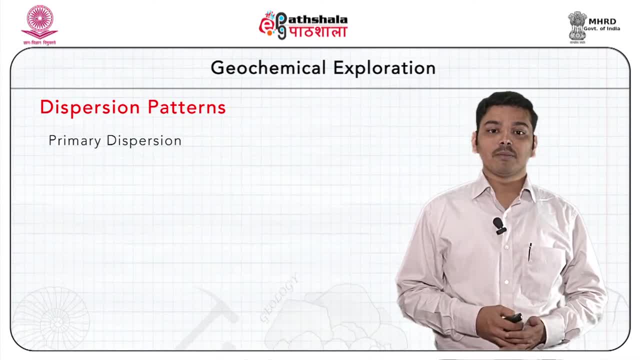 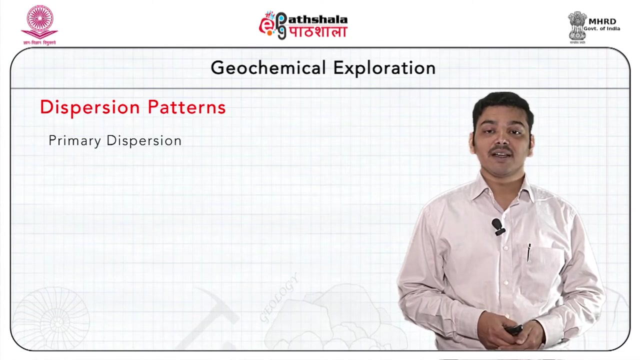 Primary dispersion. Primary patterns form at depth by igneous and metamorphic processes. The processes operative at depths of the earth are quite different from those under surficial conditions. In deep-seated conditions, relative stability of minerals under prevailing pressure and temperature conditions controls the geochemical processes. 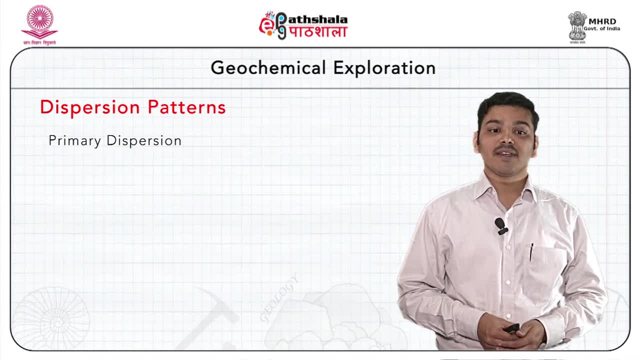 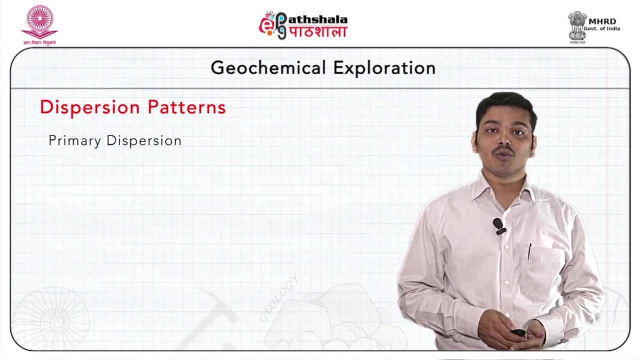 Elements entering the crystal lattice of stable mineral phases become immobile. However, those which cannot do so remain in the mobile medium until they reach an environment where they get a stable surface. Here they get accommodate in a stable mineral phase. This basic rule is applicable to all rock forming processes, whether it is metamorphism, 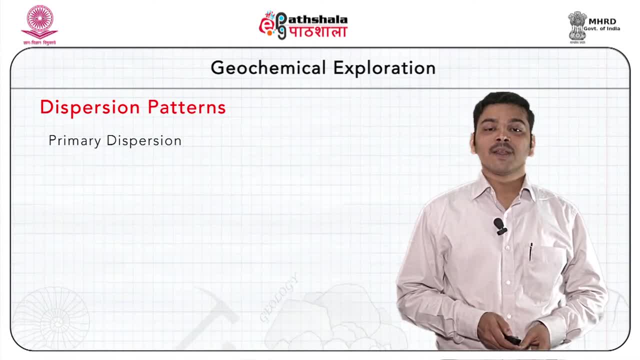 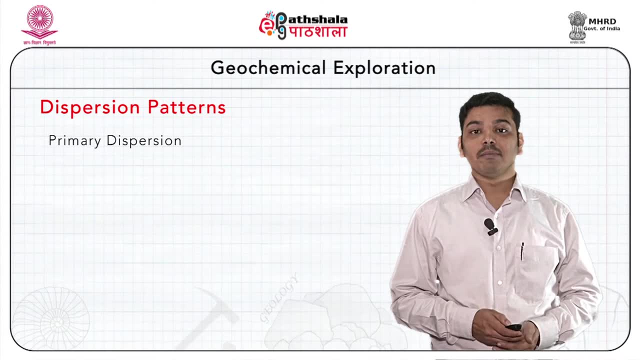 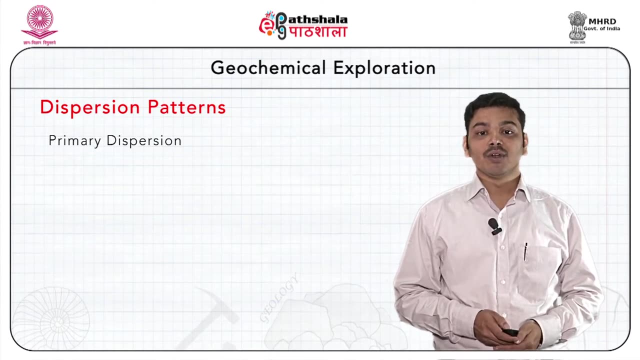 metasomatism or magma crystallization. Generally, some elements are present in abundance and thus are utilized as major constituents in the most common rock forming minerals- silicon, aluminum, iron, calcium, sodium, potassium, magnesium and titanium- in order. 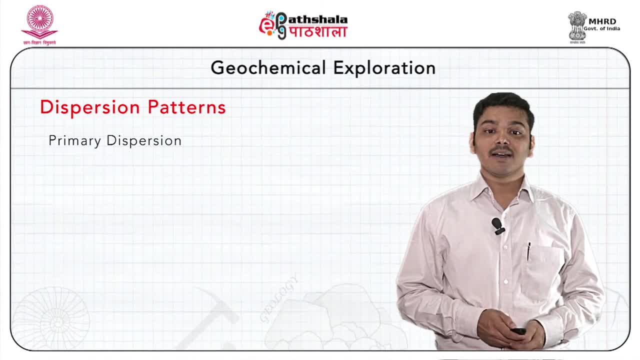 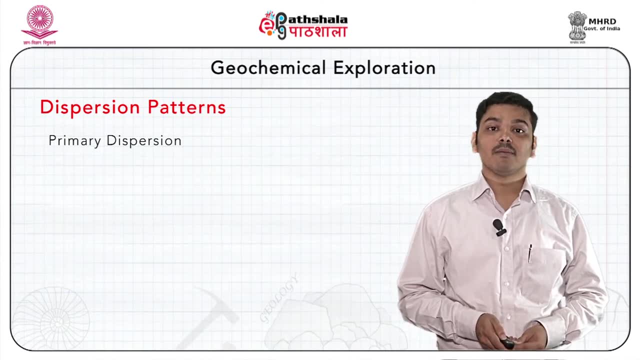 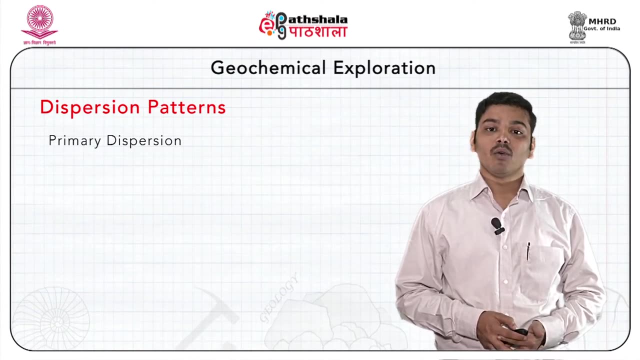 of their abundance. Rare elements occur as main constituents only in some accessory mineral phases, like zircon and monazite. The remaining elements get partly accommodated in ore or more of the common minerals by occupying a position in the crystal lattice that is generally filled by one of the major elements. 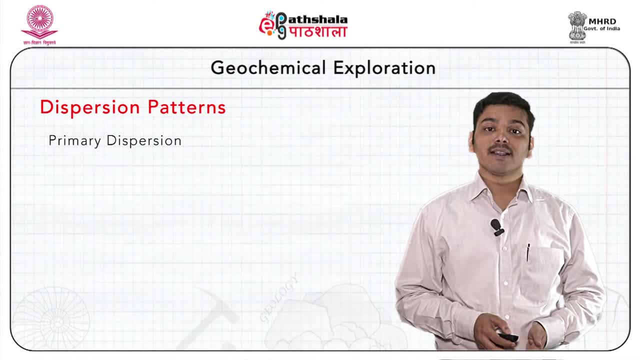 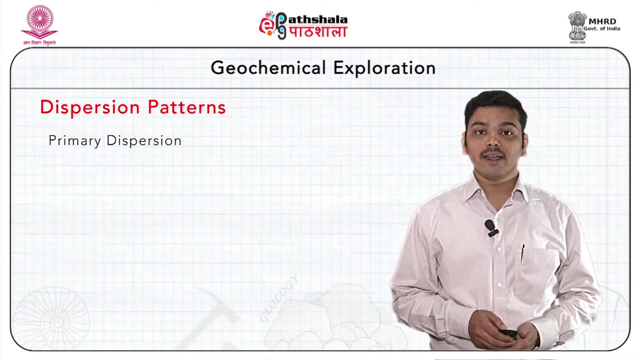 This substitution is only possible under restricted conditions. As an example, lead has an ionic radius and ionization potential close to that of potassium. Hence lead can partly substitute for potassium in potash feldspar. Similarly, zinc, copper and cobalt may proxy for iron and magnesium in biotite and amphibole. 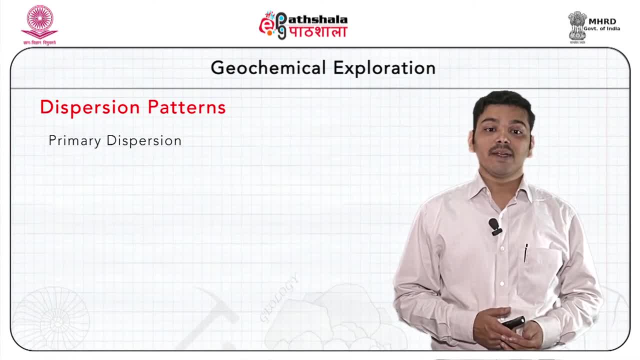 It is believed that abundance of rare elements in minerals of this kind is proportional to their relative mass. Thus there is relative abundance in the medium from which crystals were formed. In the lattice structures of rock-forming minerals, some elemental constituents cannot be accommodated and thus are concentrated in the residual medium. 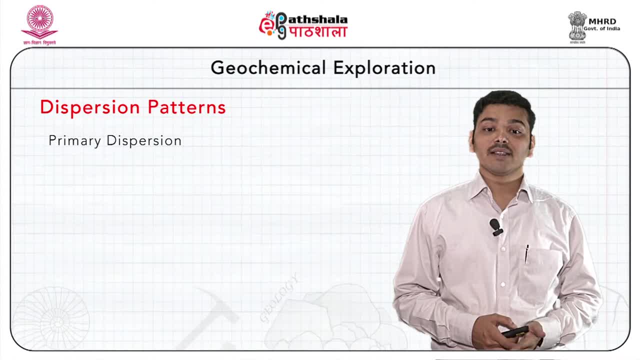 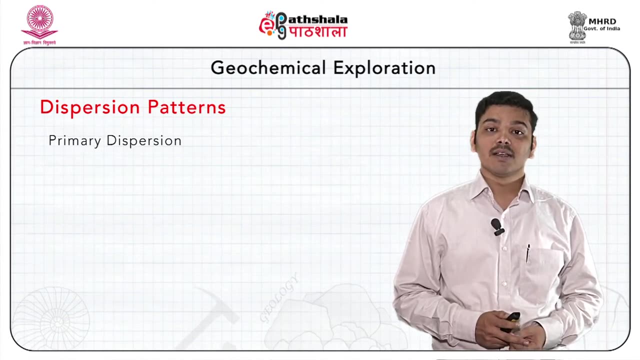 This progressive enrichment in the residual phase facilitates the formation of rare element-bearing minerals. 1., 2., 3., 4., 5., 6., 7., 8., 9., 10., 11., 12.. 13., 14., 15., 16., 16., 17., 18., 19., 20., 21., 22., 23., 24., 25., 26., 27., 28.. 29., 30., 31., 24., 24., 25., 26., 26., 27., 27., 28., 29., 29., 30., 31., 32., 32.. 33., 33., 34., 34., 35., 36., 36., 37., 38., 38., 39., 39., 40., 40., 41., 42., 42.. 43., 44., 45., 46., 46., 47., 48., 49., 50., 51., 52., 52., 53., 54., 53., 54., 55.. 56., 56., 57., 58., 59., 60., 61., 62., 62., 63., 62., 63., 62., 63., 64., 63., 64.. 64., 65., 65., 66., 66., 67., 67., 68., 68., 69., 69., 69., 70., 70., 71., 72., 72.. 73., 73., 74., 74., 75., 76., 75., 76., 77., 77., 78., 78., 79., 79., 80., 80., 81.. 82., 82., 83., 83., 84., 84., 85., 86., 87., 86., 87., 88., 89., 90., 92., 92., 93.. 92., 93., 95., 96., 97. 0. 0. 0. 0. 0. 0.. 22. 22. 23. 23. 24. 24.. 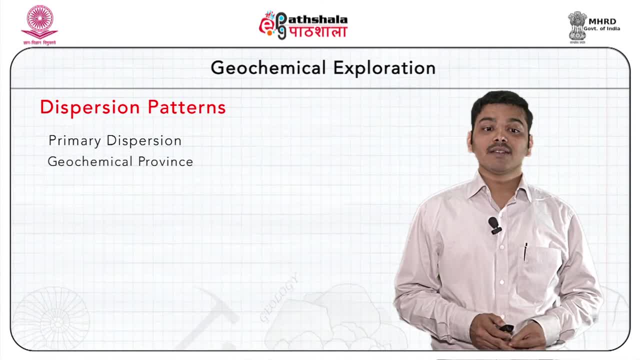 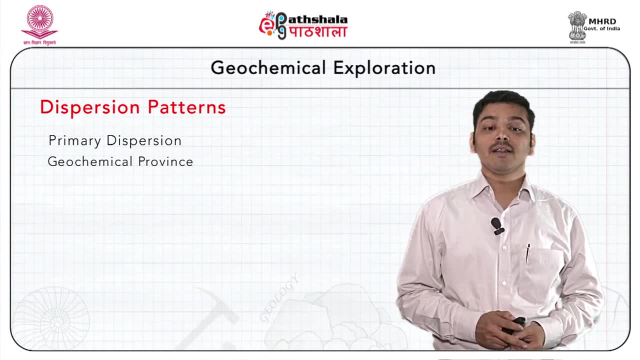 25., 26., 24., 25., 23., 26., 27., 28., 29., 31., 33.. ben dimensions 37.. flow pattern or path Based on geometry. primary dispersion patterns resulting. 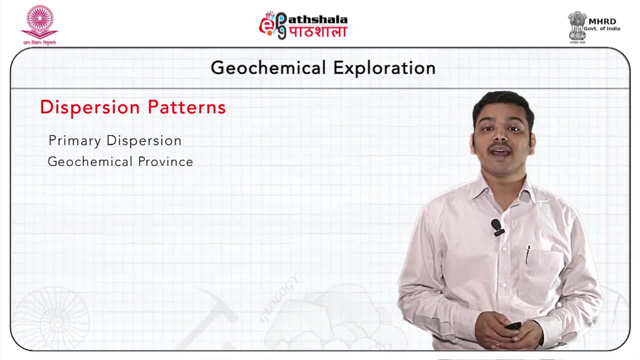 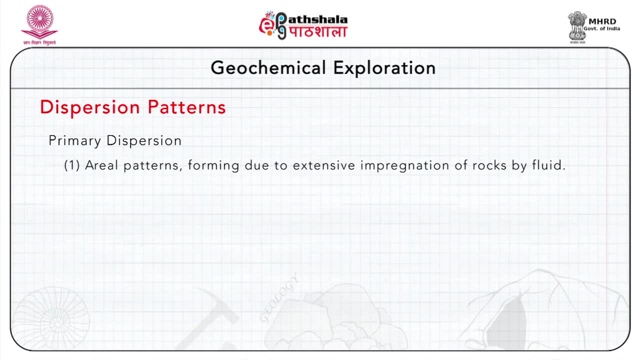 from hydrothermal fluid movement can be classified as aerial patterns forming due to extensive impregnation of rocks by fluids. second, leakage patterns formed by well-defined movement of fluids along channels, or else wall rock patterns, where the minor element composition of rock adjoining the solution channels has. 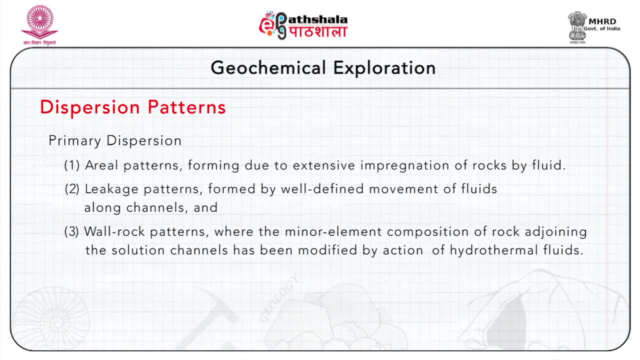 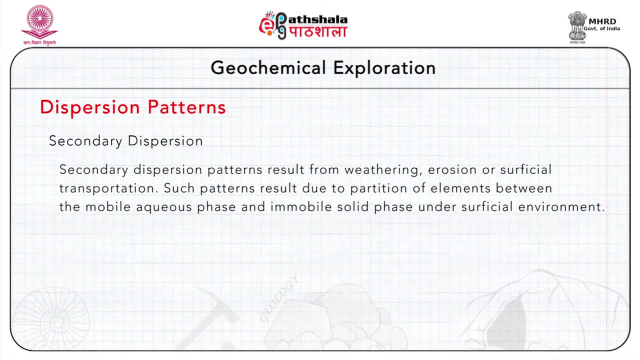 been modified by the action of hydrothermal fluids. Now the case of secondary dispersion. Secondary dispersion results from weathering, erosion or surficial transportation. Such patterns result due to partition of elements between the mobile aqueous phase and immobile solid phase under aqueous phase and immobile solid phase under. 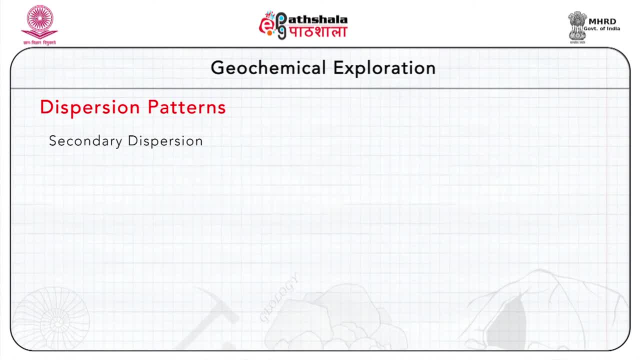 surficial environment. The resulting dispersion patterns are controlled by a number of factors or agencies which influence the pattern of material movement on Earth's surface. Secondary patterns are further categorized as halos, fans and trains, in accordance with the shape of the pattern and its 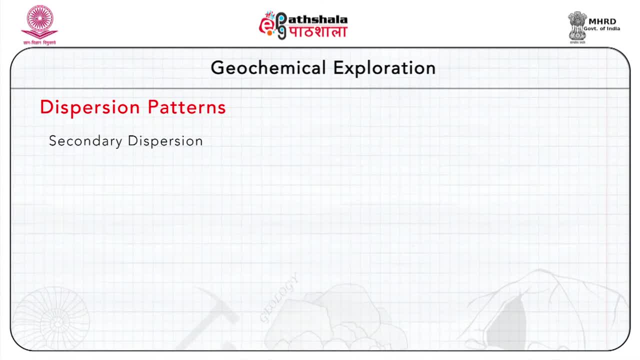 geochemical relationship with ore deposit. A halo is more or less equidimensional dispersion pattern enclosing the source of material. A fan represents the pattern of spreading outward in one direction from a well-defined source. A train is a linear pattern of dispersion caused by movement along a definite path, say a drainage channel. 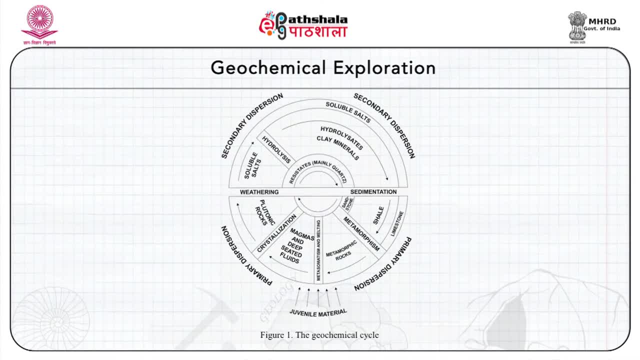 Weathering. the first phase of secondary geochemical cycle is dominated by physicochemical changes necessary to bring rock in equilibrium with new conditions on Earth's surface. Products of weathering undergo physical and chemical changes as they are transported from source regions to the site of sedimentation. The dispersion pattern of elements. 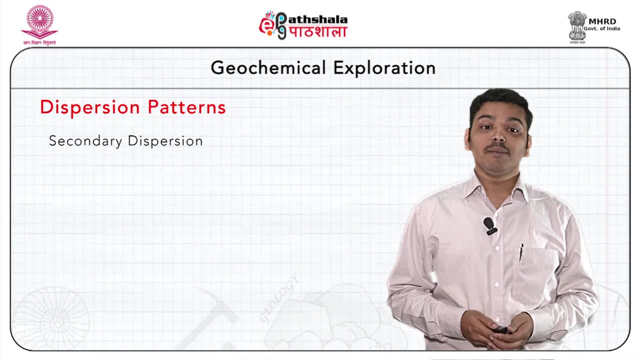 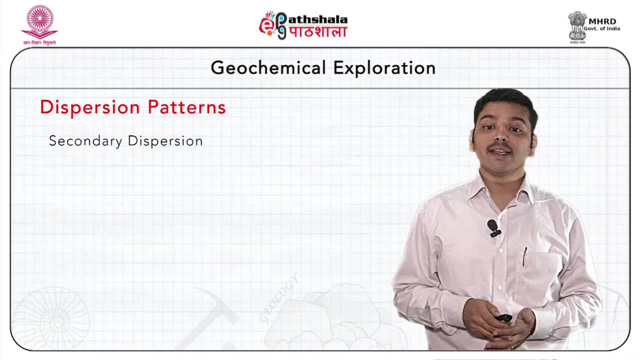 is determined by the pattern in which transporting medium, such as ice or water, moves through the soils, down drainage channels and through circulating system. It is important to understand the weathering process and various kinds of dispersion patterns generated in response to movement of weathering products. Weathering includes the mechanisms by which parent rock is. 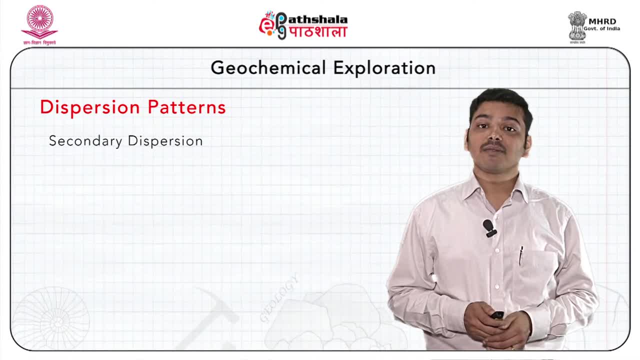 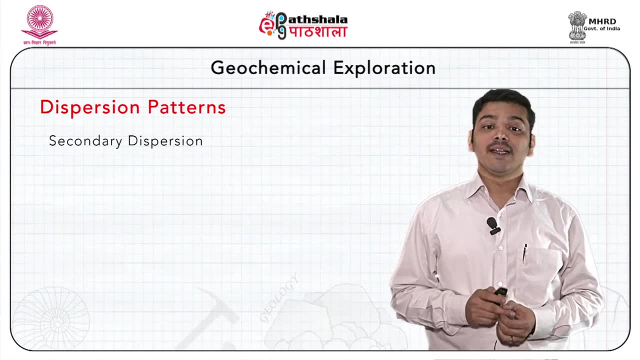 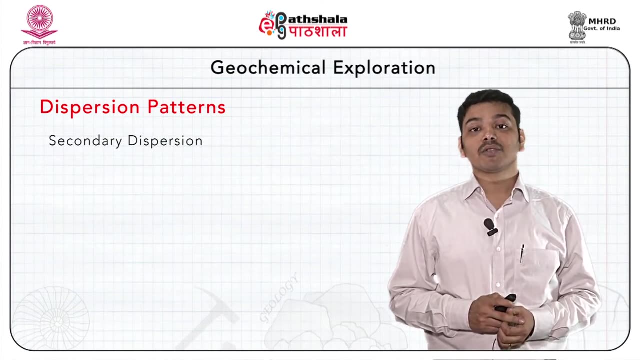 fragmented and the minerals stable in subsurface conditions are reconstituted to form new minerals stable in surface environment. Disintegration of massive rocks into successively smaller fragments dominates the physical process of weathering As against purely physical processes. chemical weathering is probably. 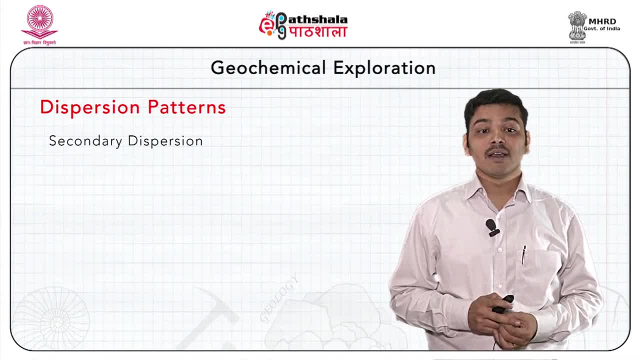 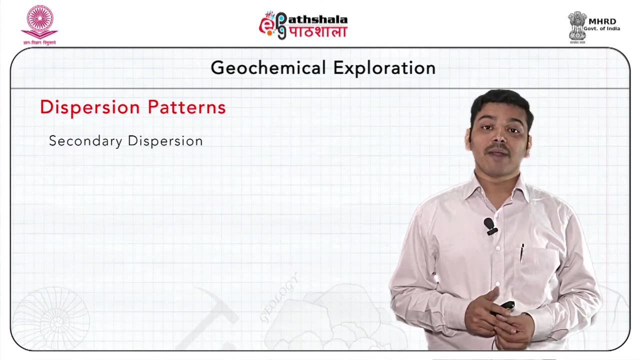 far more effective in disintegrating rocks by means of chemical reactions of rocks with abundant water, oxygen and carbon dioxide available in surface environment. Weathering products could be residual, primary minerals, secondary minerals formed at the site of weathering or soluble. 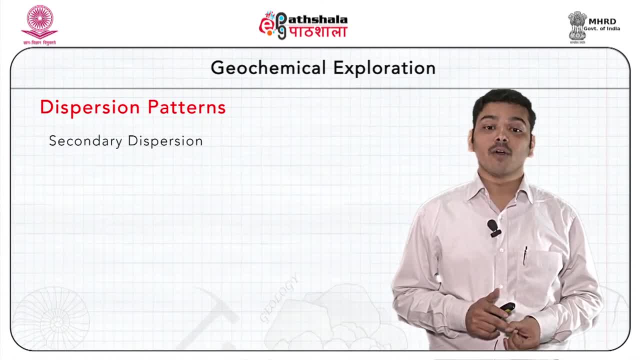 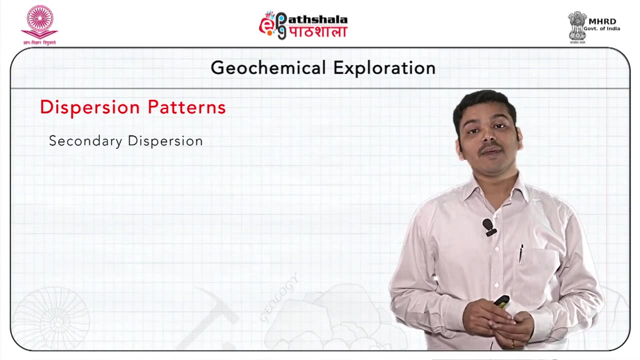 material removed from the local site by circulating water. Residual minerals are rock-forming minerals which are stable in surficial conditions or react slowly and are thus not appreciably broken down. Some of them include clay minerals, muscovite and some. 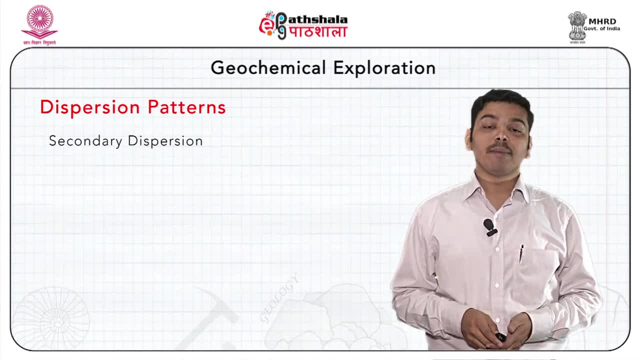 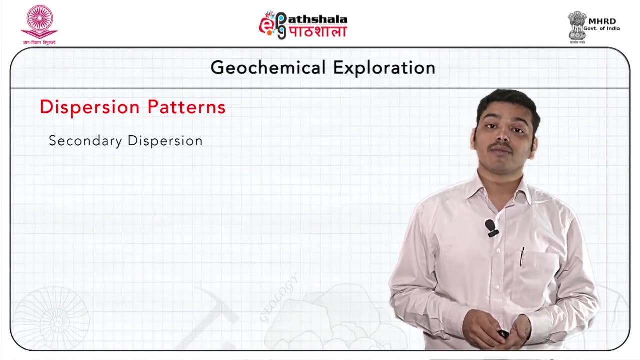 repeatable materials such as FeClAlS, Strange Ayurvedic contraceptives- preserve, restore alive day-to-day quality minerals in large, large quantities of chlorites. Secondary minerals are mainly the products of hydrolysis of primary mineral constituents of rock undergoing weathering. Clay minerals and few hydrosilicates such as chlorite and vermiculite are source of the secondary minerals. 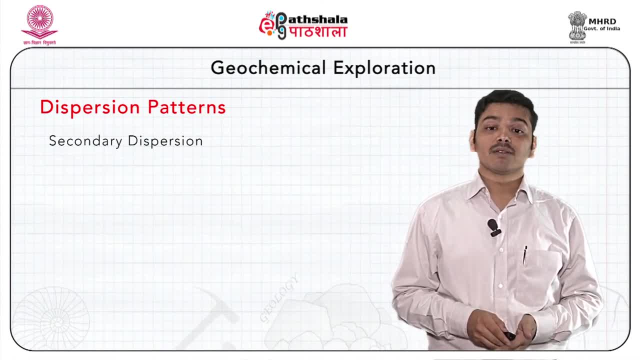 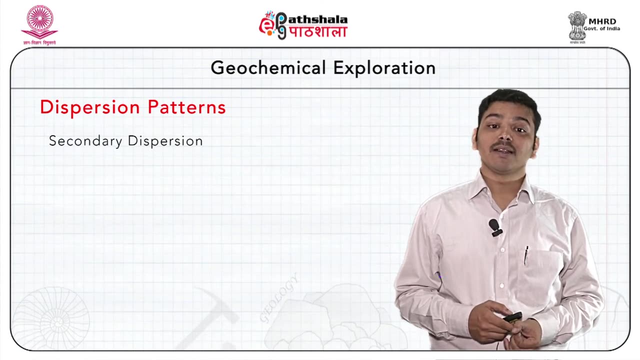 The physicochemical environment of weathering strongly influences the suit of secondary minerals. The soluble products of weathering comprise those constituents which are released by the decomposition of primary minerals and are not required to form new suit of secondary minerals. Lime and magnesia may be soluble products for calcareous rock. 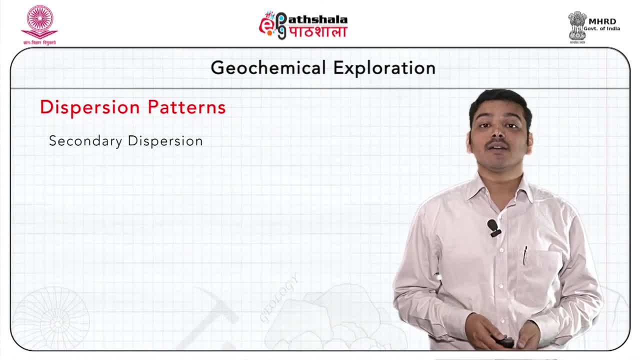 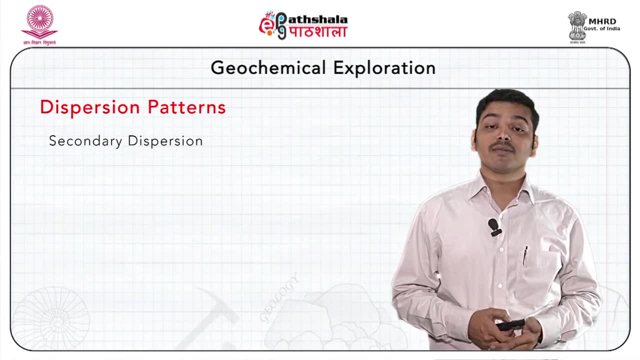 However, for granite soda and potash could be the dominant ones. The relict patterns of resistant minerals are often considered as important result of secondary dispersion During weathering. some primary minerals in rocks and ore bodies are not completely disintegrated. 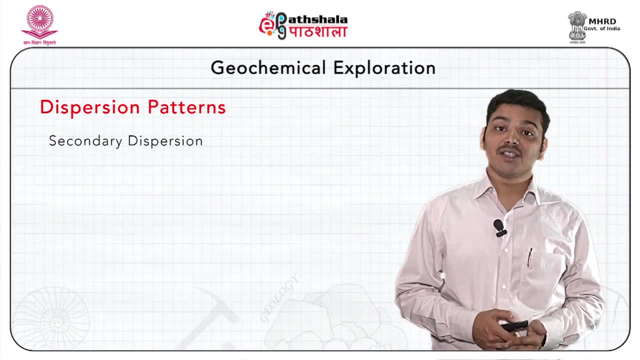 If such minerals have unique association with its original host. qualitative mineralogical analysis of the residual soil could be critical to determine the identity of parent rock or ore. The pattern of mineralogy can be used to determine the identity of rock or ore. The pattern of mineralogy can be used to determine the identity of rock or ore. 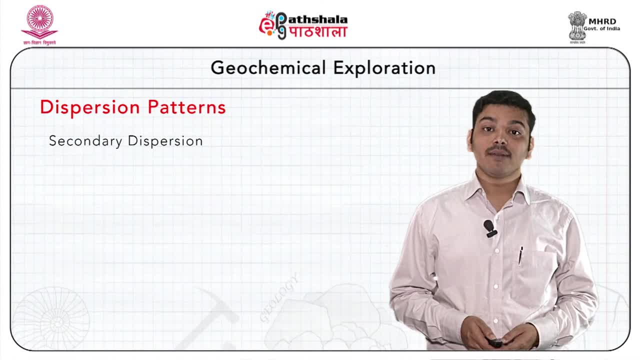 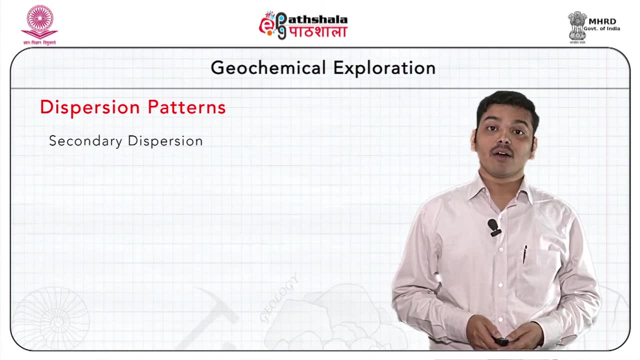 The pattern of secondary mineral in residual cover is also helpful to identify the nature of parent rock In deeply weathered regions. the color of soil is one of the important yardsticks for geologists to ascertain the nature of parent rock. The color of soil depends on the limonite content, a secondary mineral reflective of iron content in the parent rock. 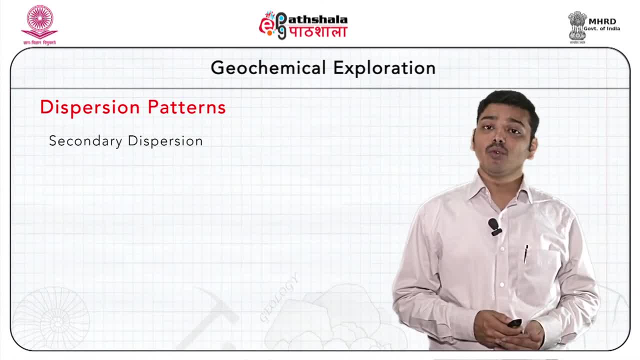 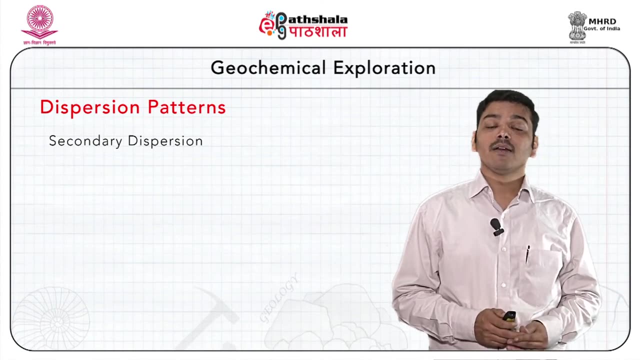 In some residues, minerals may be too fine-grained for easy identification. Thus, chemical analysis of residual material is needful to identify the chemical signatures inherited from parent rocks that are not evident from casual investigations. Analysis of soils for trace elements is widely used and is a successful method of geochemical exploration. 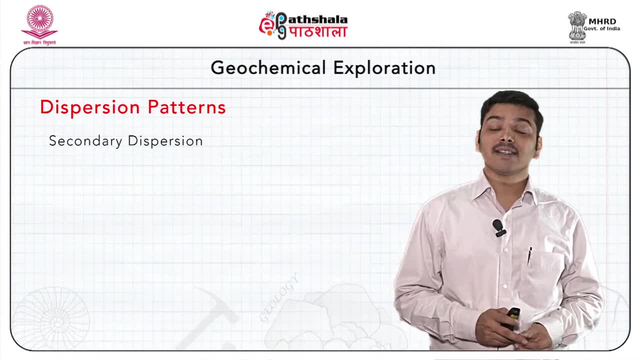 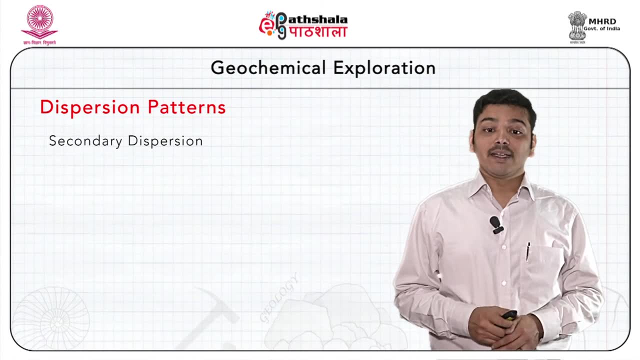 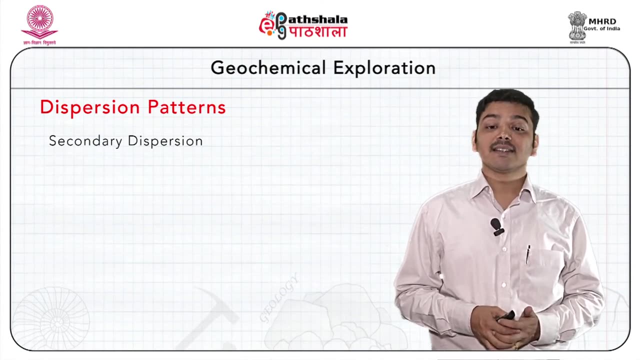 The absolute metal content in soil as against that in the parent rock depends on the mobility of metal. As an example, even if an ore body may contain similar concentrations of lead and zinc, lead shows relatively immobile nature, as against zinc that tends to be leased out. 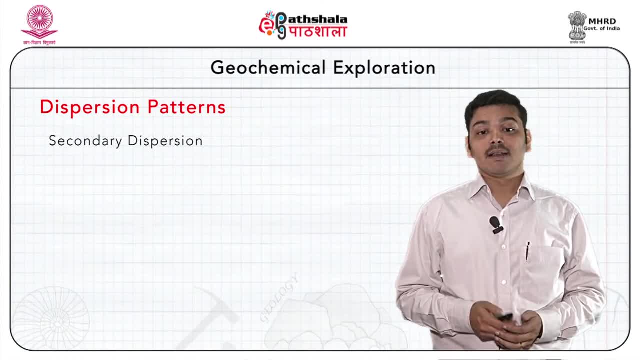 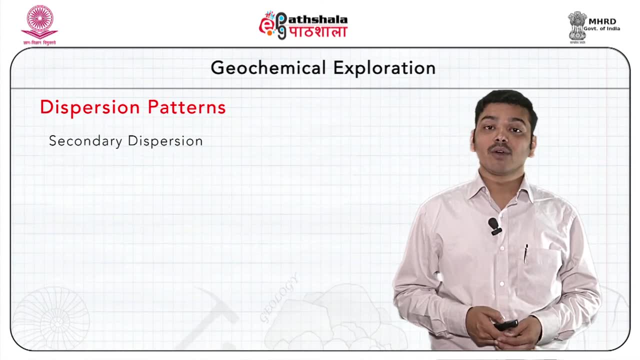 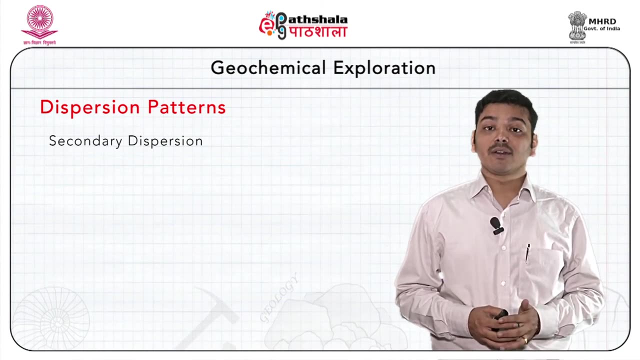 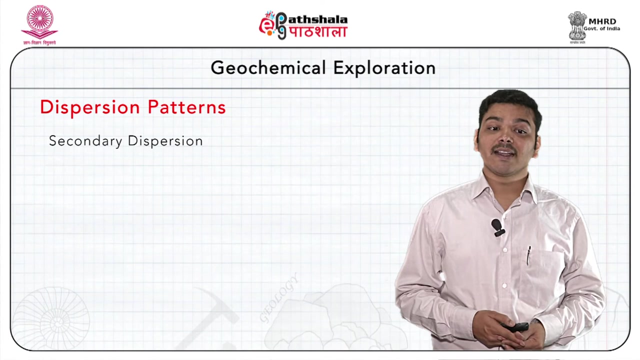 Although a major part of mobile metals are removed from the site of weathering, a significant part may degrade, get relocated in close proximity by weathering. A significant part may just get relocated in close proximity by transporting solutions where it may re-precipitate. The resultant is a lateral and downhill spreading of the 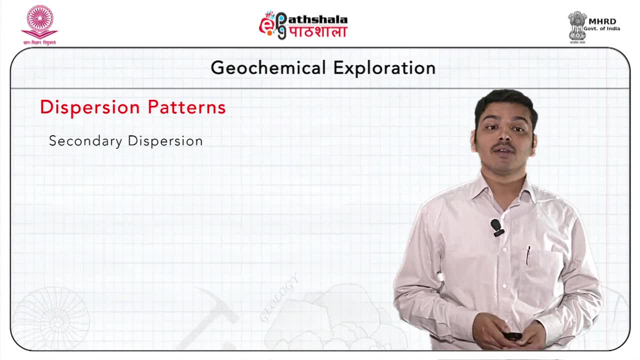 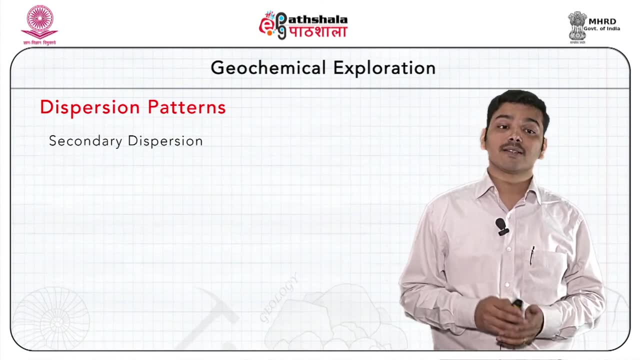 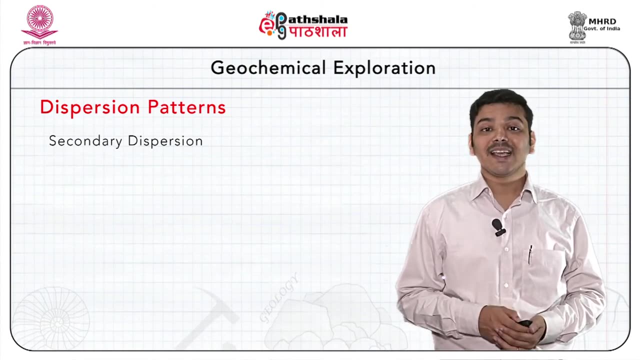 dispersion pattern outward from the source. rock Mobility of metals also constraints the homogeneity of a metal pattern in residual soils. Mobile metals such as zinc may form a characteristic homogeneous pattern. This indicates that the original erratic variations in distribution of metals in soils tend to 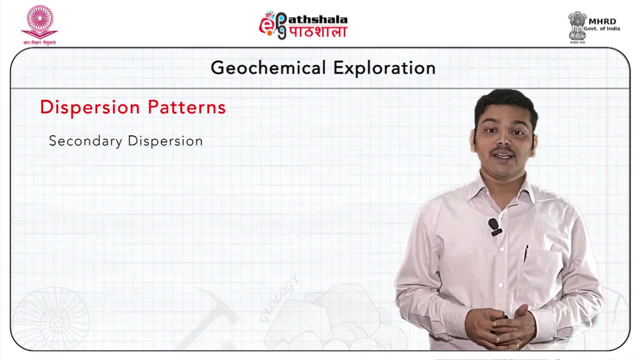 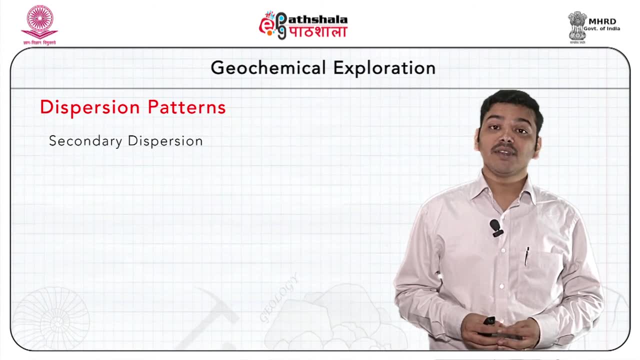 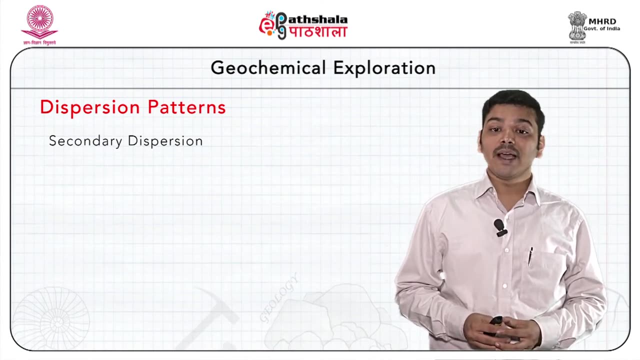 be smoothed by solution. The homogeneity of a geochemical analysis is considered important while deciding for the most efficient spacing of samples in practical surveying, As against anomaly developed by immobile metals, fewer sampling points are needed to locate and map an anomaly formed by 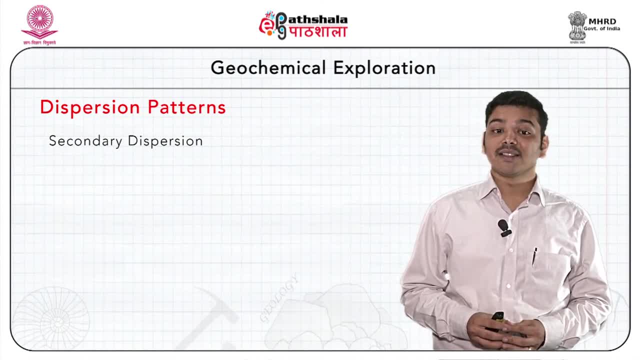 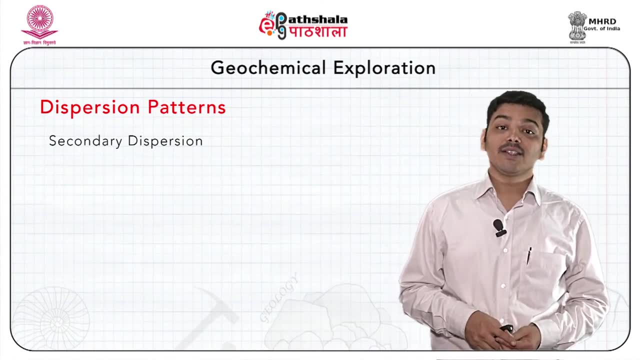 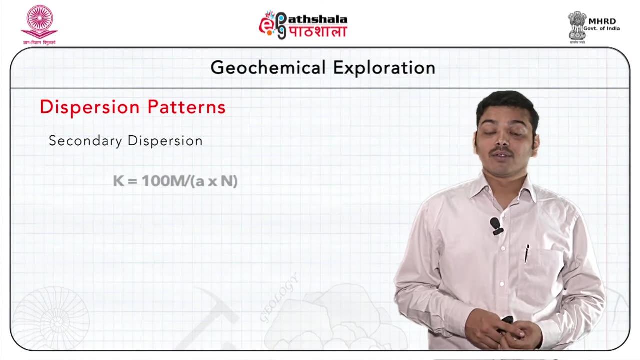 mobile metals. The coefficient of aqueous migration, which is denoted by the symbol K, is a measure of the mobility of elements. This is the ratio of the concentration of an element in dissolved solid and in associated rock. So K is equals to 100 M divided by multiplication factor. 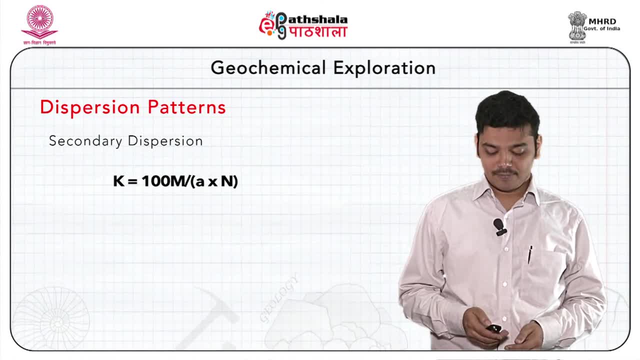 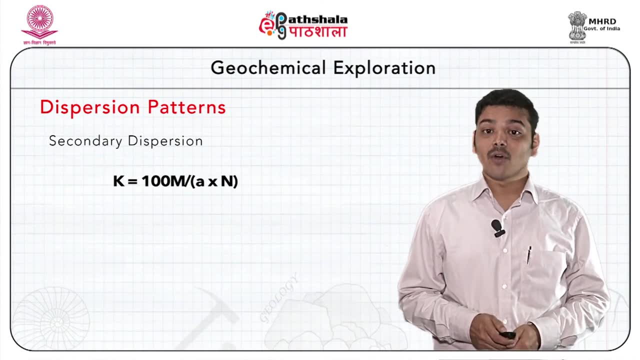 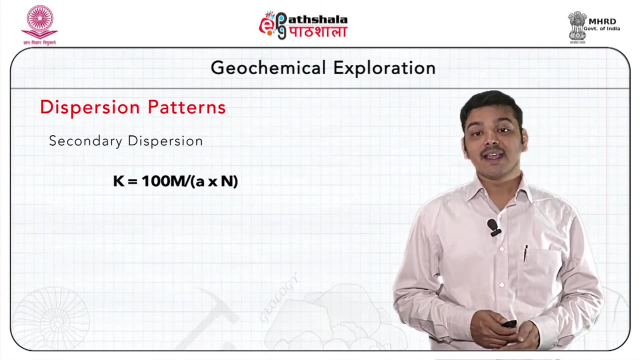 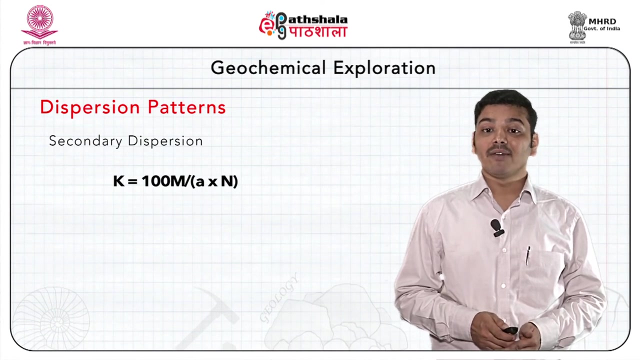 of A and N, where M is the concentration of element in drainage waters in milligrams per liter, A is the total mineral residue in water in percentage and N is the concentration of element in rocks, again in percentage. The parameter K varies for an element from oxidizing to reducing. 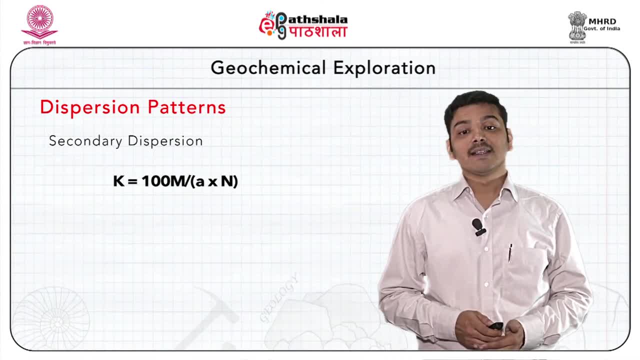 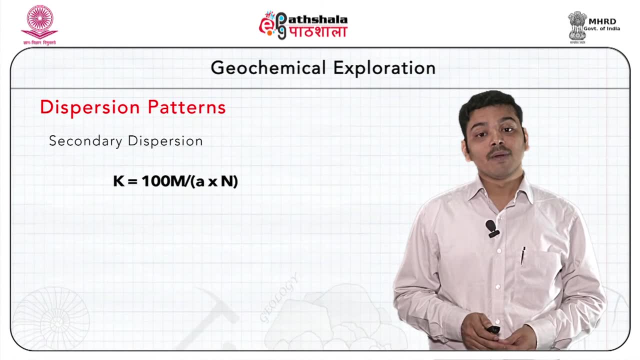 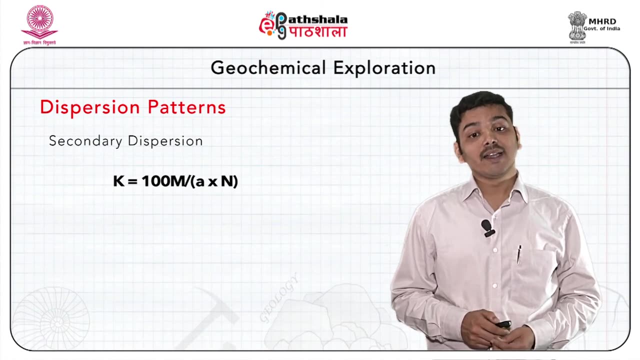 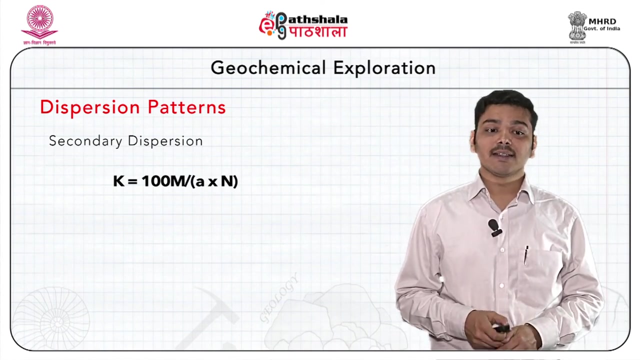 conditions. The Hawkes model relates strength of an anomaly to grade and size of ore bodies. He showed that in a mineralized zone trace element concentration of stream sediments could be linked to area of drainage basin above the sample location. background concentration of element and the area and concentration of trace elements in soil anomaly overlying an. 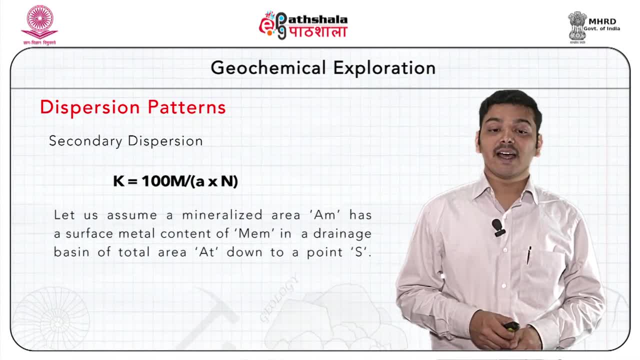 ore body. The H is the total mineral residue in water in percentage and N is the total mineral residue in water in percentage and N is the total mineral residue in soil. anomaly overlying an ore deposit. Let us assume a mineralized area A-M has a surface metal content of M-E-M in a drainage. 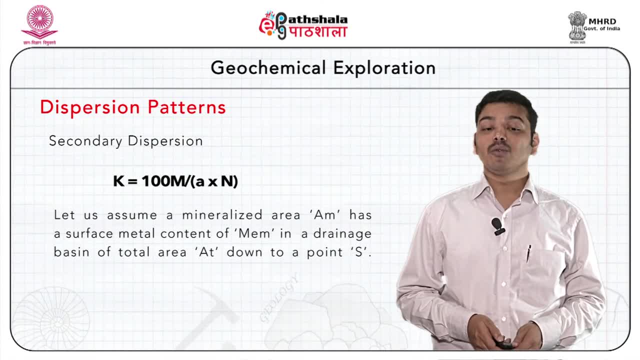 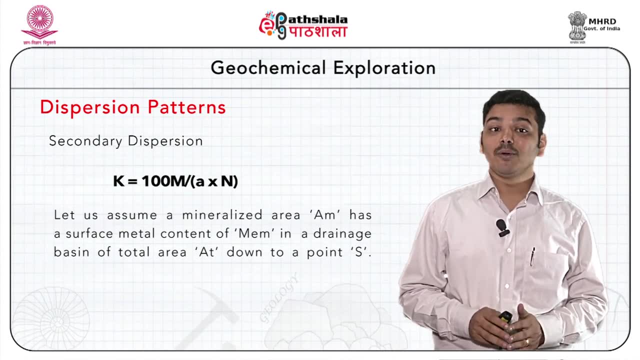 basin of total area A-T down to a point S. The background metal content is assumed to be M-E-B. that is contributed from barren tributaries and erosion of barren bank materials. If erosion processes remove material from all parts of the drainage basin, it is assumed to be M-E-B. 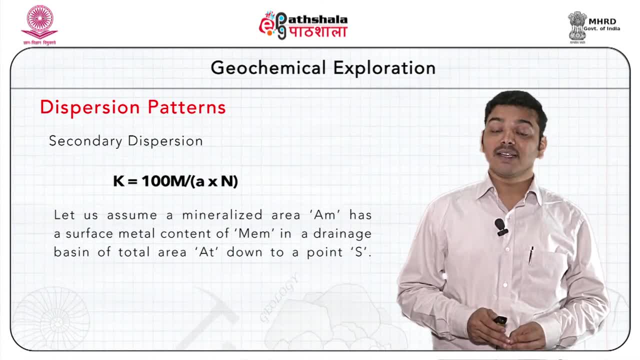 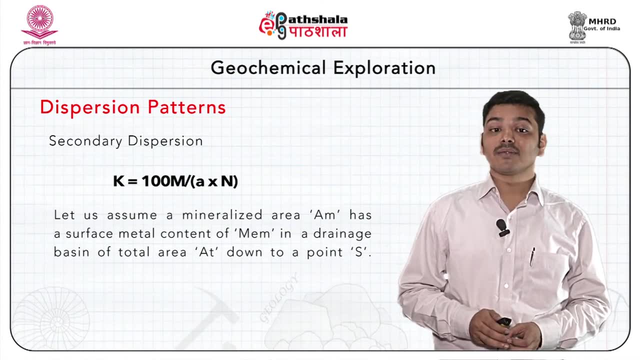 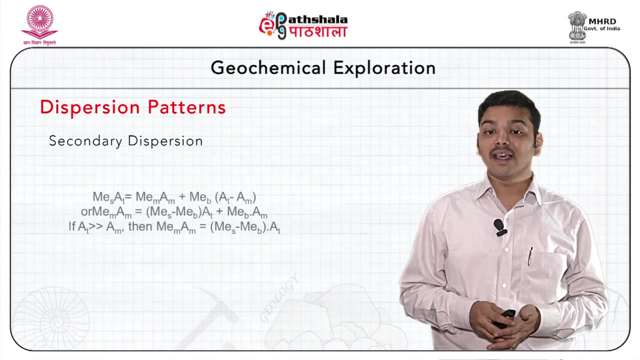 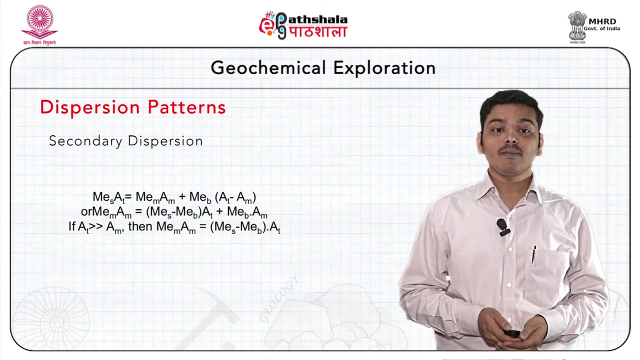 So what is the main difference between this restriction of the sediment content at point S and the sediment content of the middle basin at point S? cán be expressed as shown in the equation in your text. Thus, M-E-A-M is the measure very. 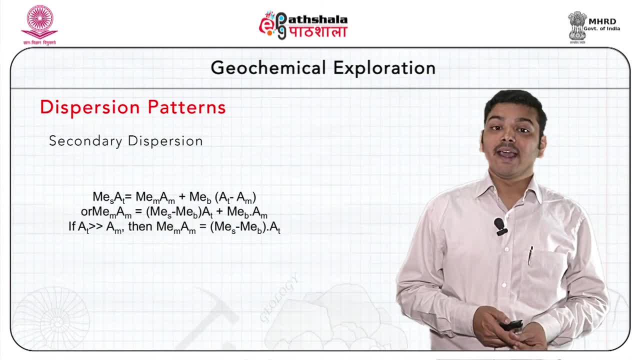 larger than the size quantity feels. However, there is a major difference between the two Kingdom of the deposit or source and MES minus. MEB is a measure of the strength of anomaly above the background. Hence the exposed size and grade of source can be. 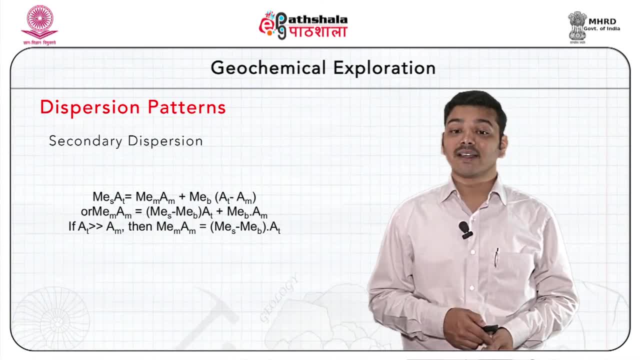 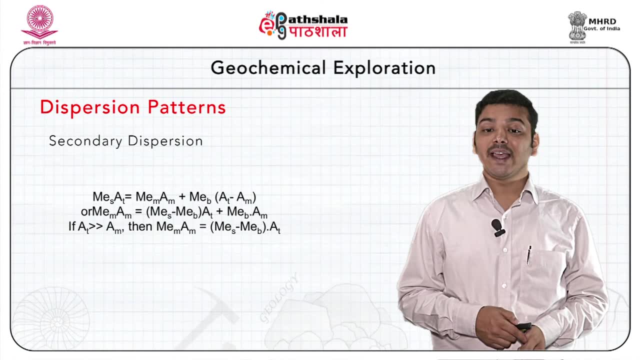 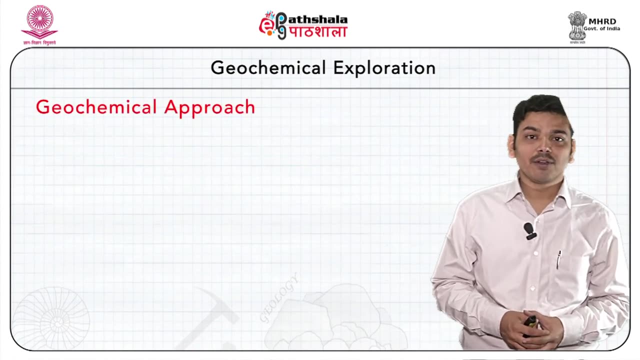 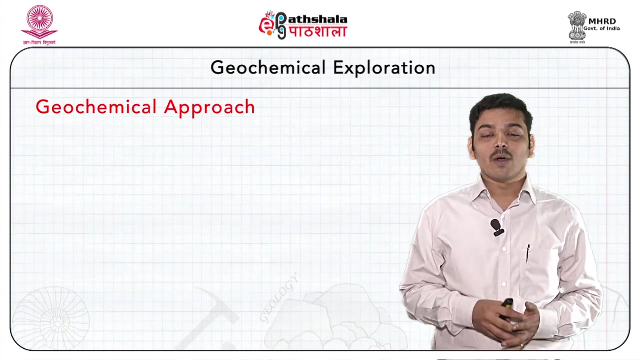 estimated from an observed value of anomaly strength multiplied by the drainage area. The quantity MES minus MEB multiplied by AT is generally termed as productivity of sediment anomaly. The next section of this module is on geochemical approach, which describes or discusses about what should be our 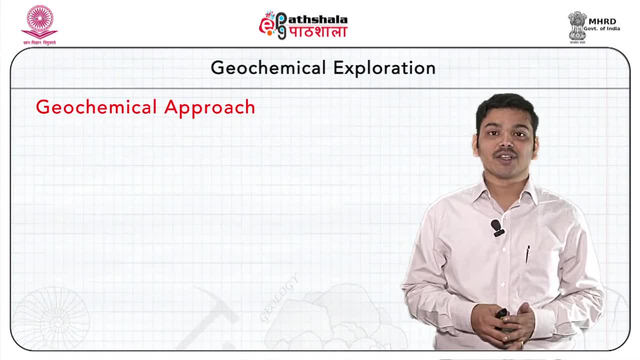 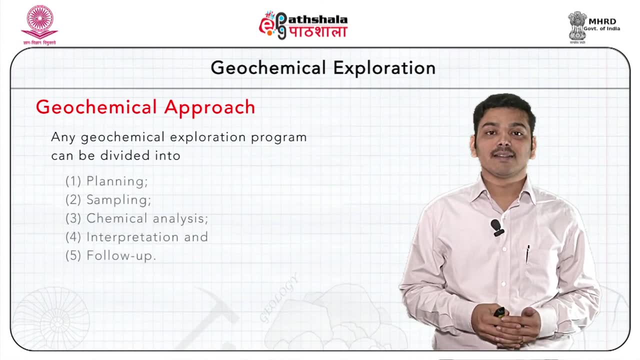 approach in any geochemical exploration program. Any geochemical exploration program can be divided into several stages like planning, sampling, chemical analysis, interpretation and follow-up. In overall, the exploration program is based on a systematic sampling. thus decision-making, analysis and evaluation Decisions need. 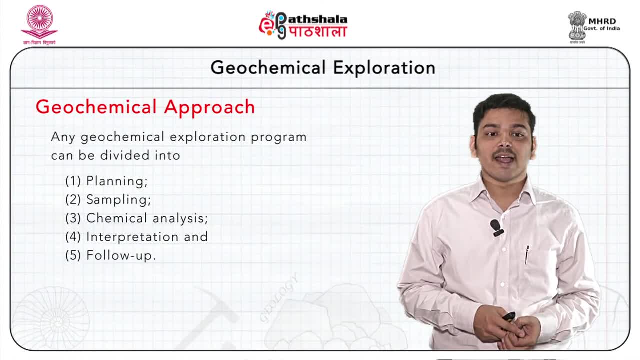 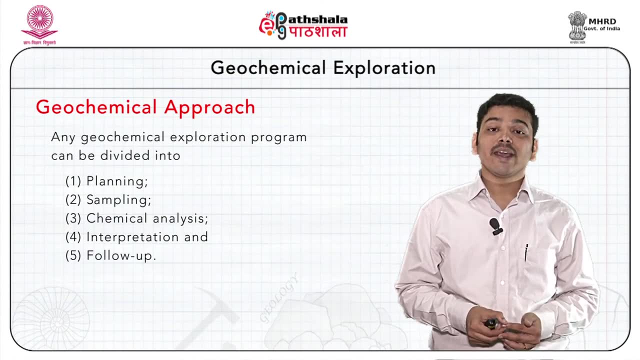 to be taken. considering some parameters like cost, nature of material samples and density of samples, in addition to analytical technique, It is likely that a more expensive method would be the most effective. Thus, cost by benefit ratios must be considered carefully Overburden. 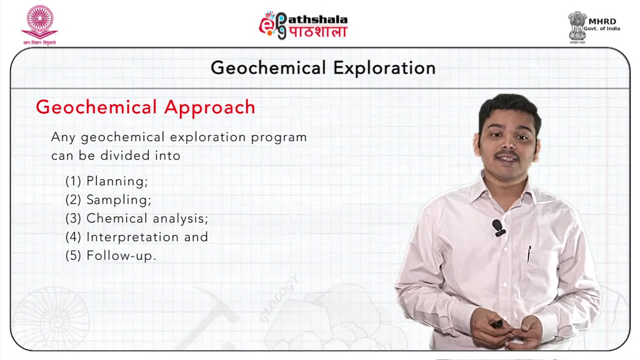 conditions are critical to determine the material to be sampled. However, density and nature of samples are important. These are mainly on the basis of previous experience in area or, if possible, an orientation survey. So in the text of this module you may go through: 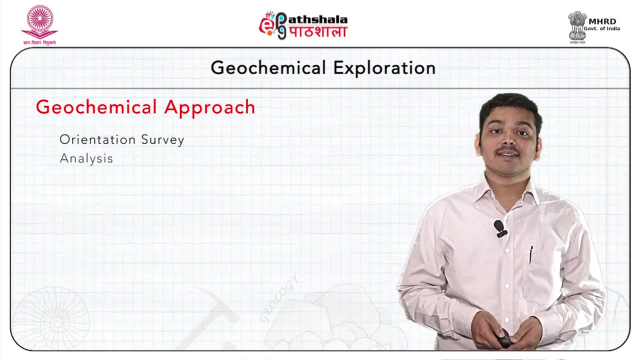 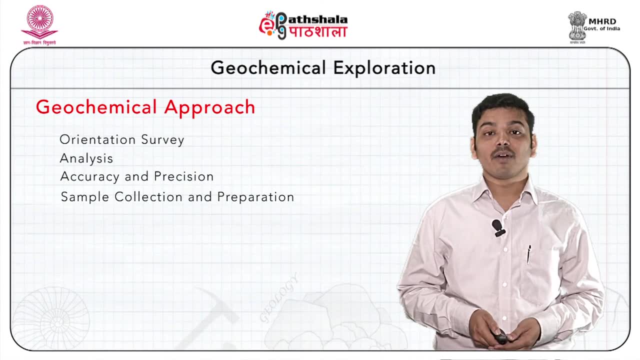 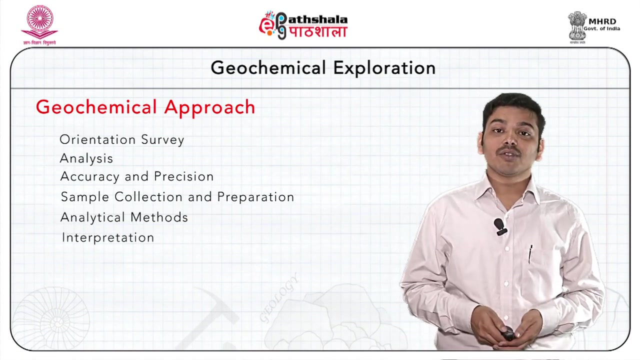 orientation, survey and analysis. what is the importance of accuracy and precision, how we should collect the sample and prepare them for further analysis, and the various analytical methods commonly employed worldwide during any research. So now coming to the interpretation part. the use of statistical analysis is 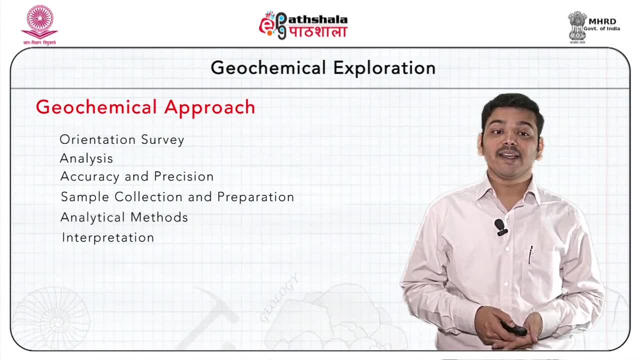 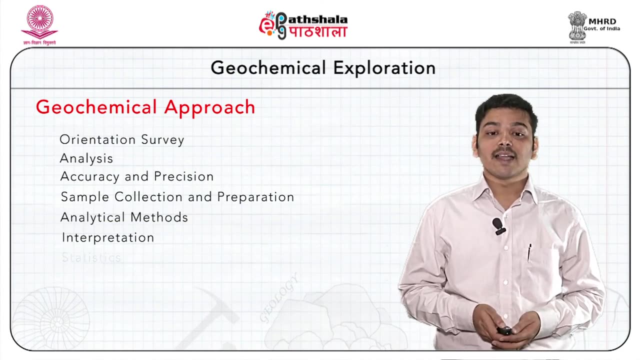 useful, as the data are likely to be multi-element and of large number of samples. Transfer of data in the form of CD-ROM or over the internet is most preferable, as paperwork is expensive and almost certain to add errors. Statistics also plays a very important role in geochemical exploration. 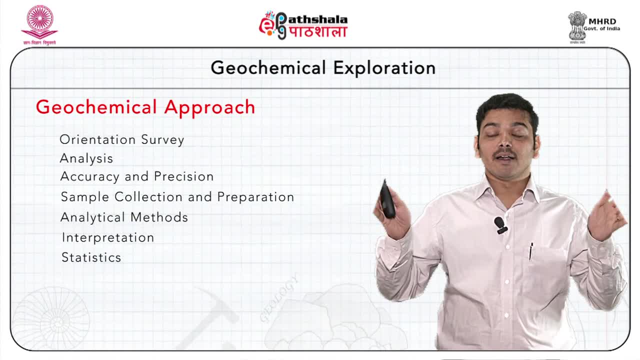 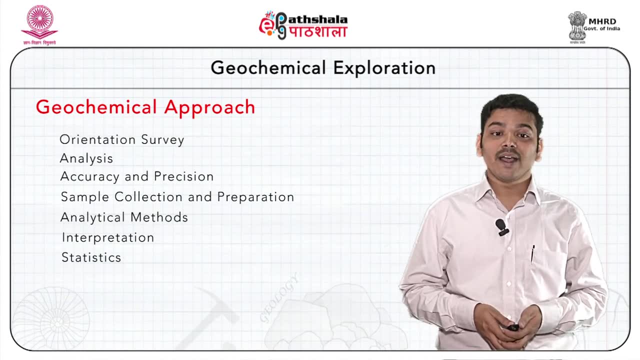 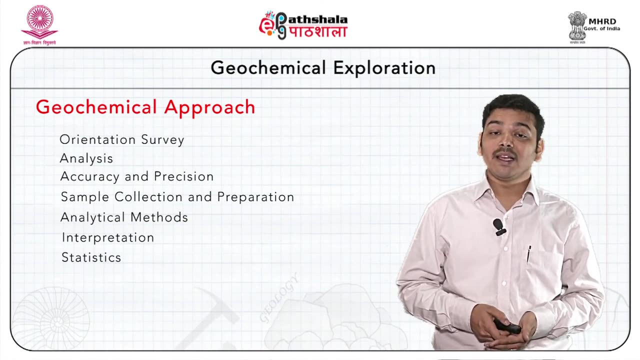 In geochemical exploration and in decoding, as well as aligning the large amount of data set we have produced. So defining significant anomalies is the main objective of geochemical exploration program, and anomalies are defined by statistically grouped data and their comparison with geology and 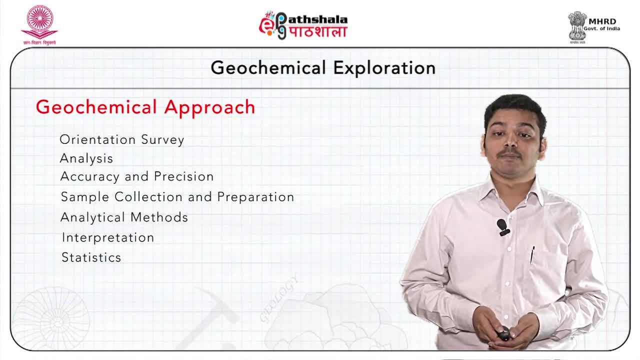 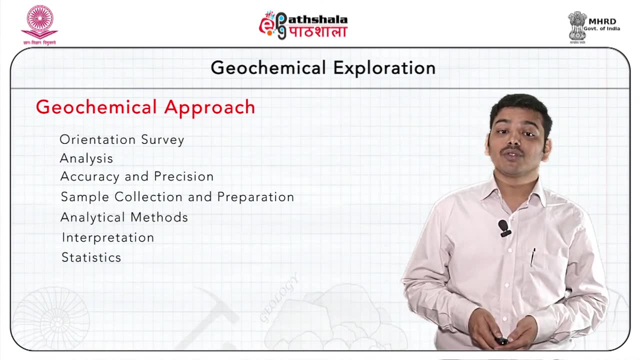 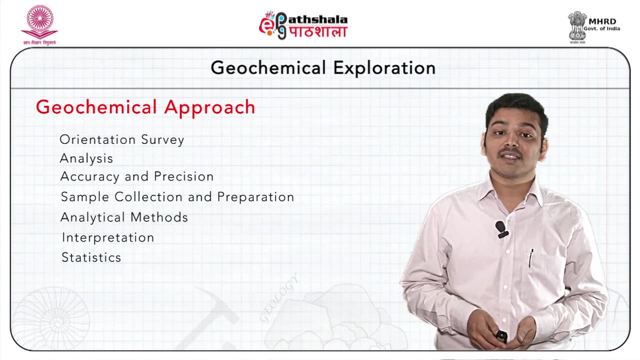 sampling information helps to interpret them. In order to compare geochemical data with geology and geophysics, the most useful final product is to summarize the data in map form using a grading or GIS package. Results of statistical analysis are combined with that of elemental mapping to define areas of 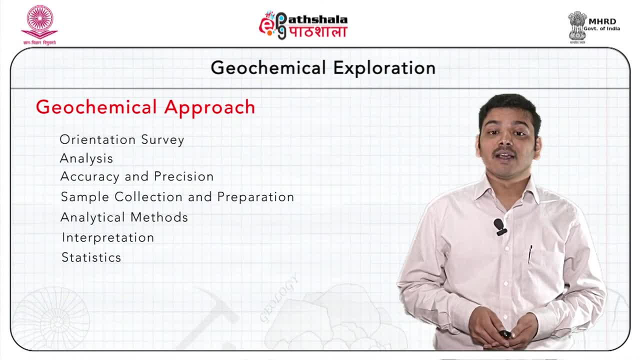 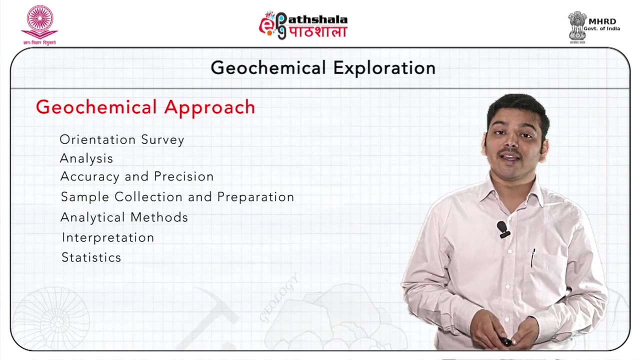 interest that demand detailed investigation, classification of such areas based on origin of chemical anomaly, seepage or probable residual anomalies. The aim of overall exercise is to produce rational exploration for chemistry of all areas of interest and not just to say that they are of unknown origin. 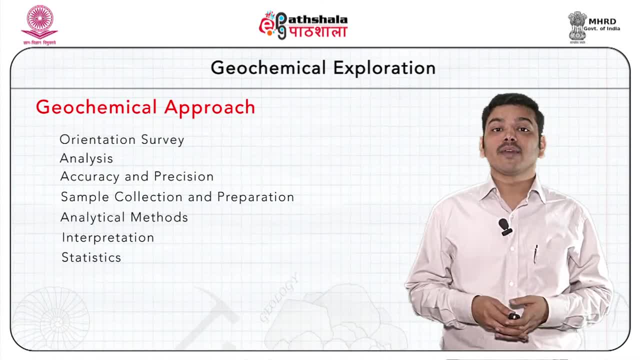 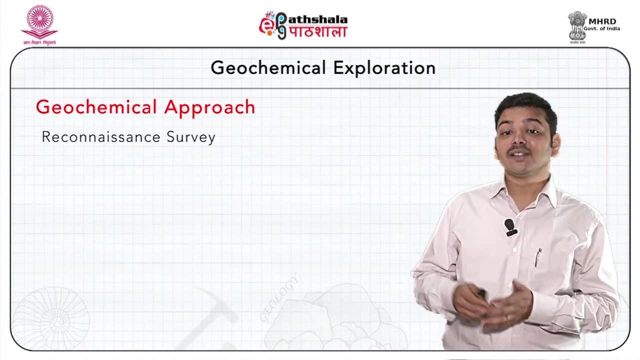 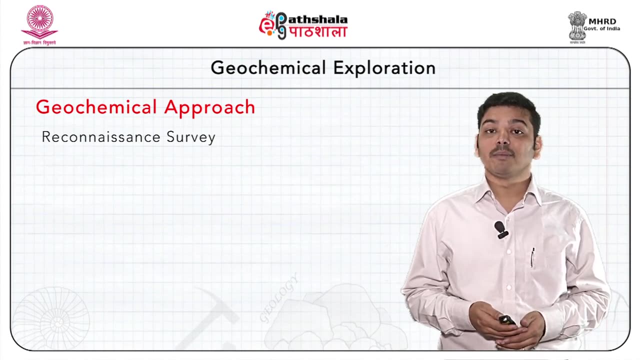 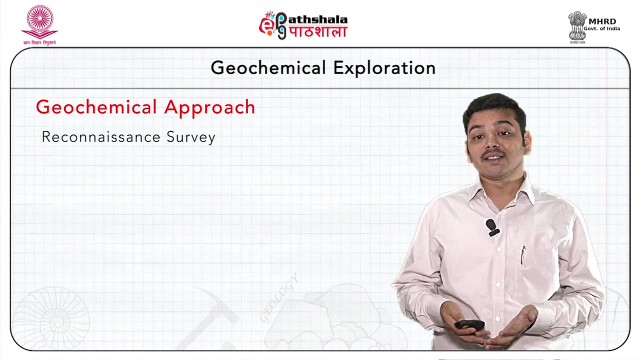 The next approach of any geochemical exploration program is recognition survey, the type of which depends on the origin of the overburden. For residual type of overburden which is derived from rock underneath, the problem is straightforward. However, in the case of overburden of exotic nature which is transported from somewhere else, different methods must be used. 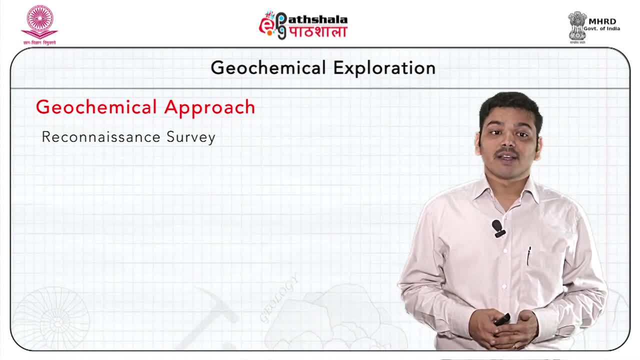 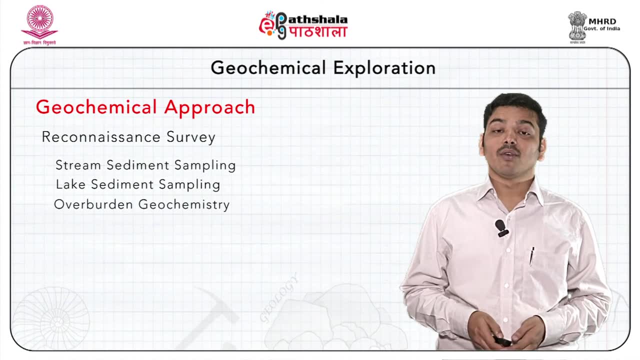 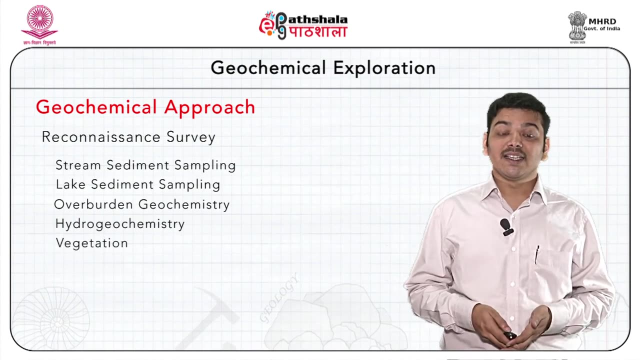 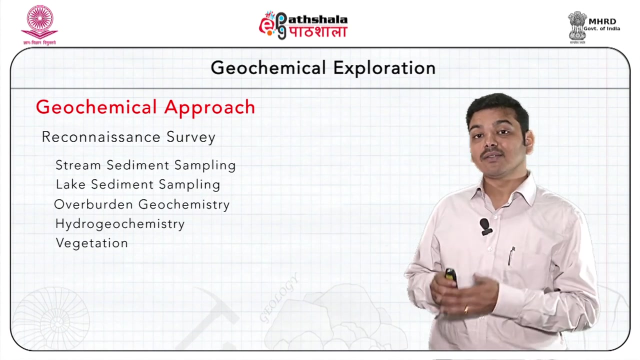 Some of the common components of any recognition survey are like stream sediment sampling, lake sediment sampling, followed by evaluation of overburden, geochemistry, Then hydrogeochemistry, understanding the nature of vegetation and its implications towards any exploration program, and this is finally eventually followed by follow-up sampling. 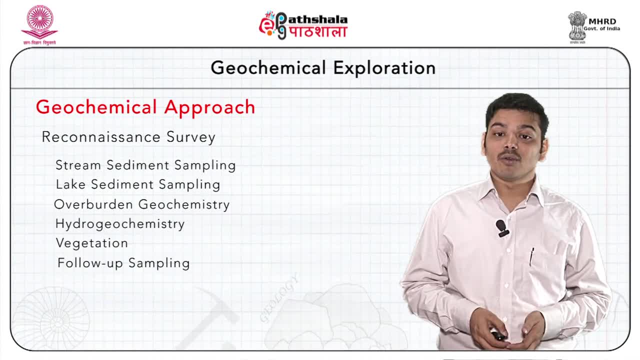 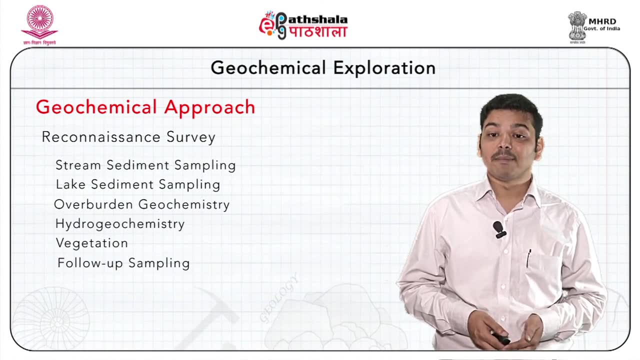 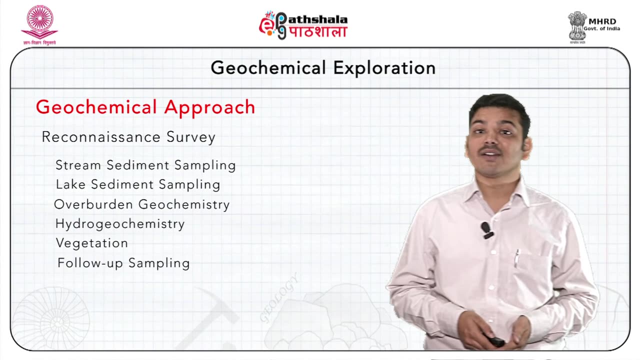 In follow-up sampling. anomalies and possible source regions identified during recognition sampling need to be defined further by detailed sampling in order to locate drilling targets. The next process is geochemistry of the rocks. In addition to sampling of the rock resistance, areas of elemental enrichment are highlighted by elimination of background areas. 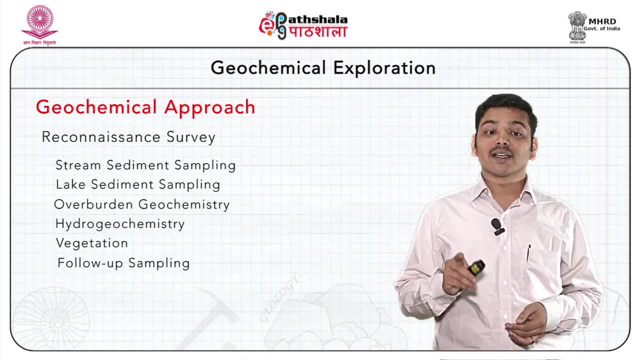 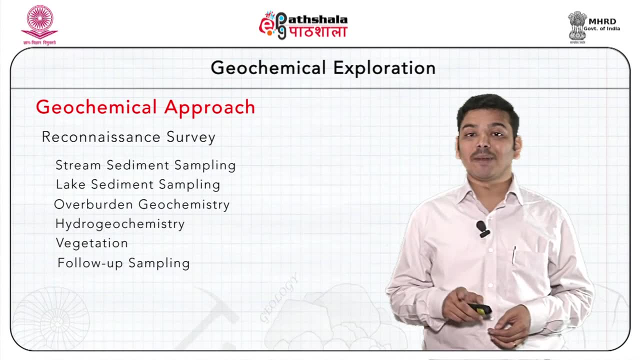 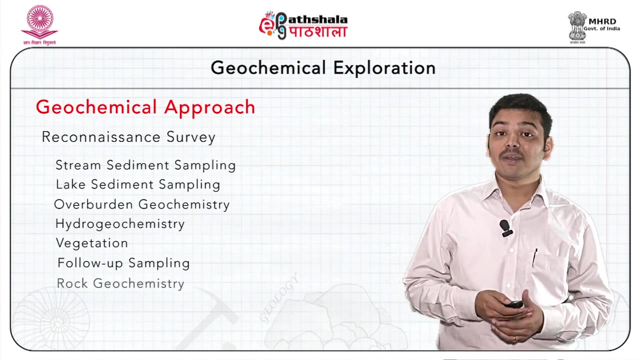 During the recognition phase, stream or lake sampling processes involves overburden sampling of the catchments. Thus, for soil or overburden sampling, follow-up process involves a denser sampling approach until the source of anomaly is identified. Next is geochemistry of the rocks. In the follow up technique, survey and observation geochemistry or ge tsunami are used to these results. Next is lifestyle geochemistry of the rock. In the follow-up techniques, all different different methods of geochamistry are used. ằp90 Seeing describes the layer and locally mixed rock partition. 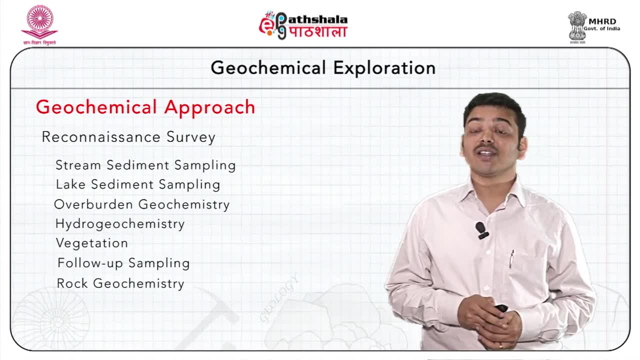 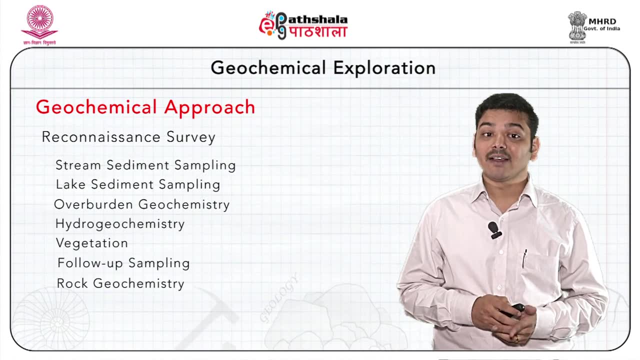 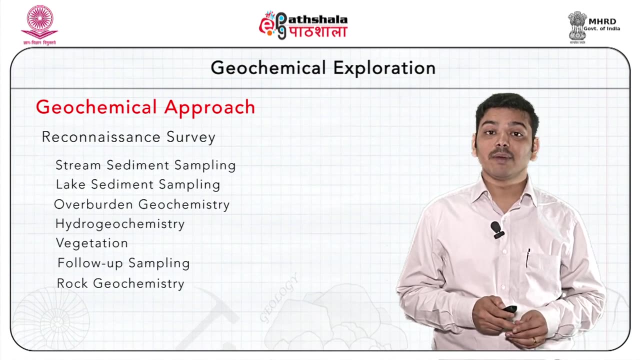 rock sampling or drill core acquisition is carried out particularly for areas of good outcrops. one needs to be careful while collecting rock samples to avoid contamination. products of surface weathering should be removed using steel brush. generally, one kilogram of sample is enough for base metal exploration. 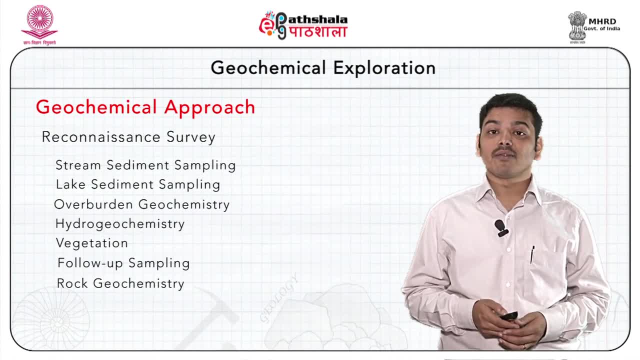 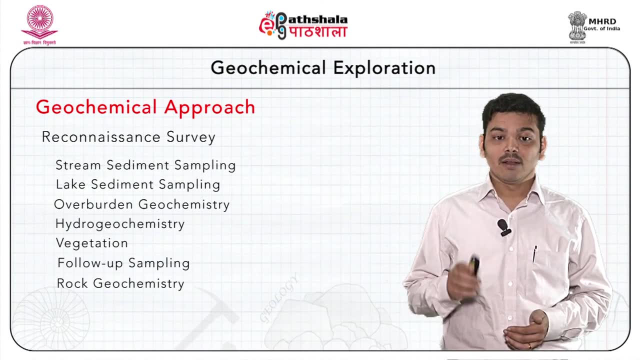 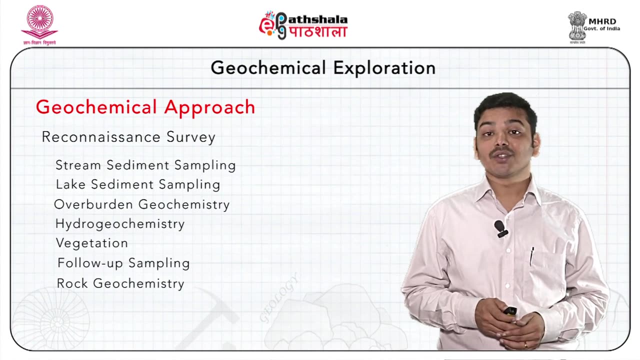 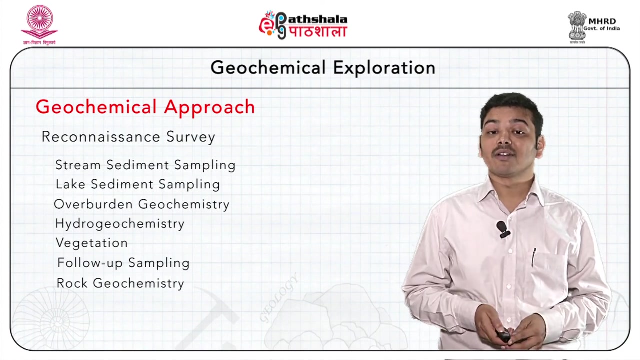 however, for precise determination of metals, especially precious metal concentrations, larger samples, possibly as large as 5 kilogram, are required. rock geochemistry depends on the interpretation of multi-element data and computer-aided interpretation, with meticulous subdivision of samples based on mythology. so, based on the discussion,